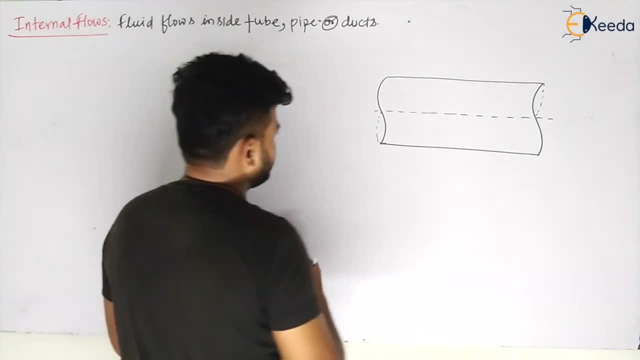 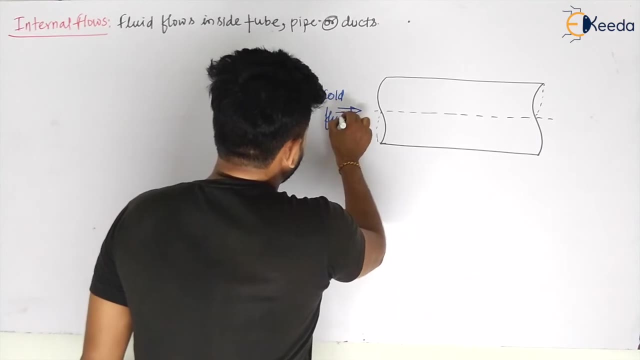 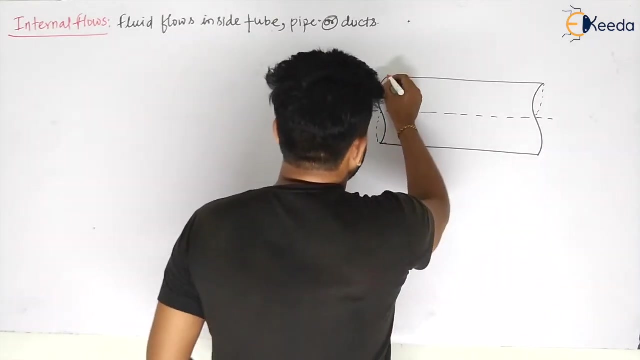 Let us say, let us say cold fluid is flowing inside the pipe. Cold fluid is flowing inside the pipe, my dear students. Cold fluid is flowing inside the pipe. Now the surface of the pipe is hot. Now the surface of the pipe is hot, my dear students. 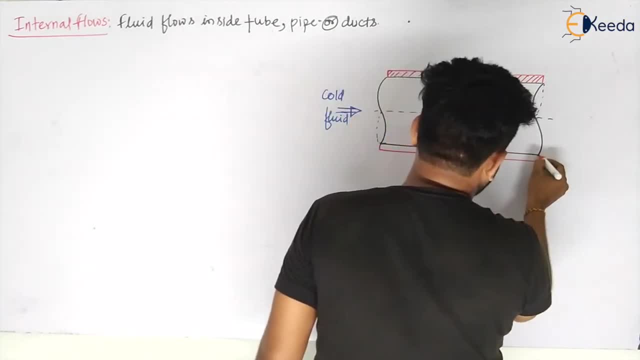 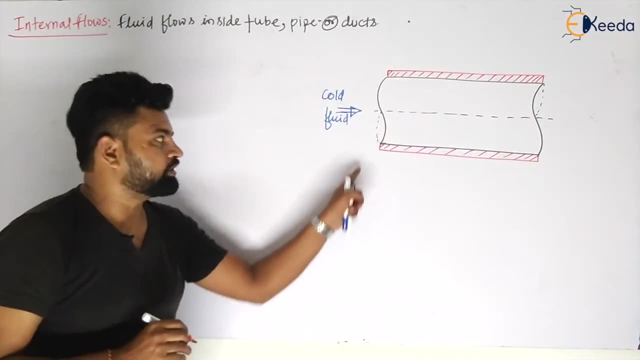 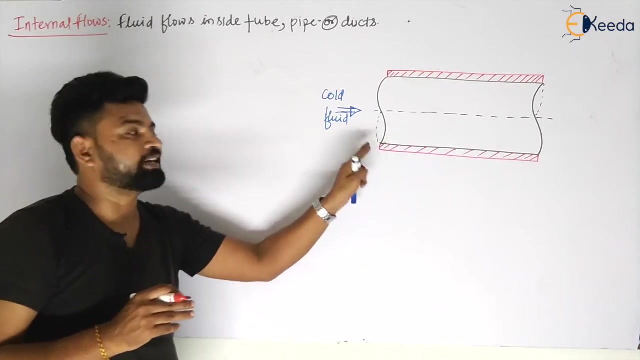 It will be hot for the both side. So, as soon as the fluid will touch this surface, my dear students, what will happen? There will be no solid condition and the velocity of the fluid will decrease And it will become equal to zero. at that point, my dear students, 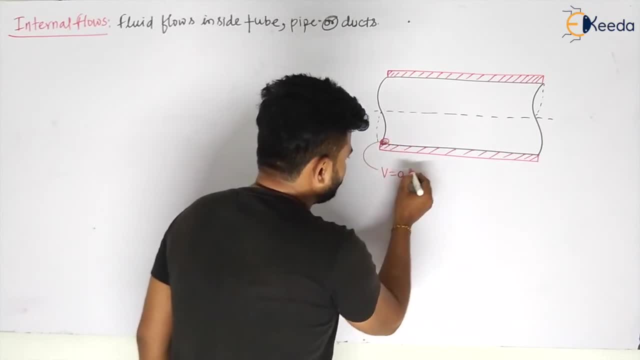 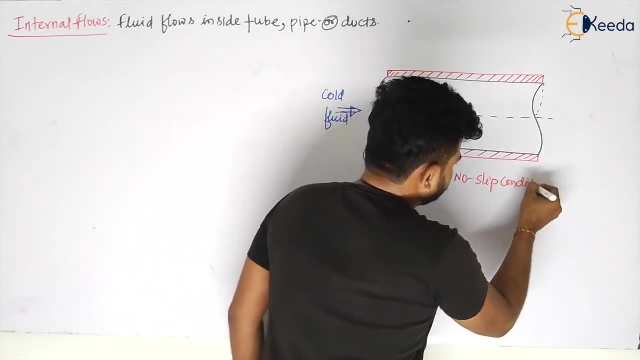 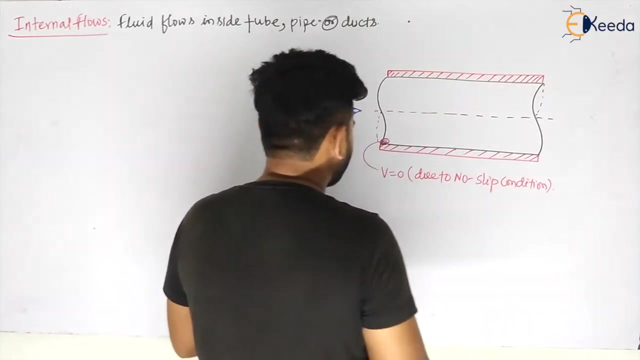 velocity of the fluid will become equal to zero. due to what? due to no slip condition. no slip condition, my dear students. okay now, due to no slip condition, the velocity is becoming zero. so what will happen? let us see what will happen. let us see, so, slowly, slowly, there will be what heat transfer from fluid, from this hot plate to. 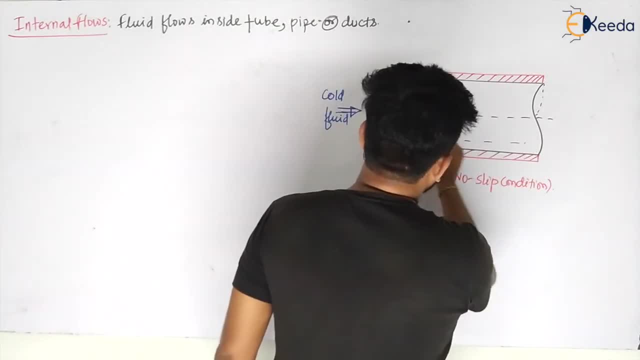 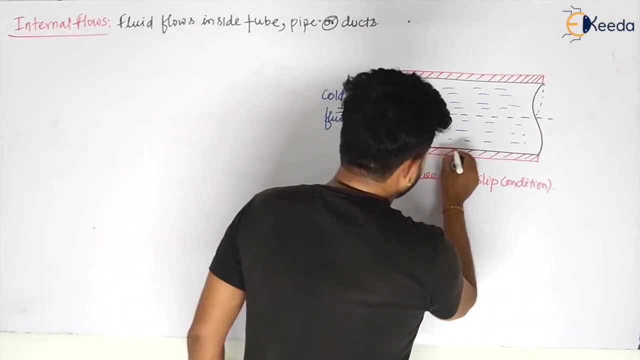 the cold fluid, my dear students, which is flowing inside this pipe, yes or no? yes, sir, there will be some heat transfer. in what direction? in the upward direction. so there will be development of what. there will be development of this like this: if TS is the surface temperature of the pipe, then what will? 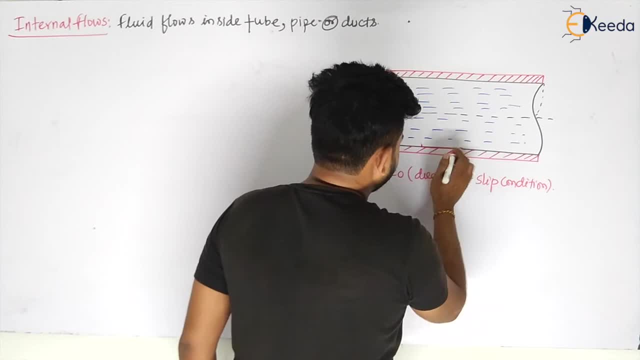 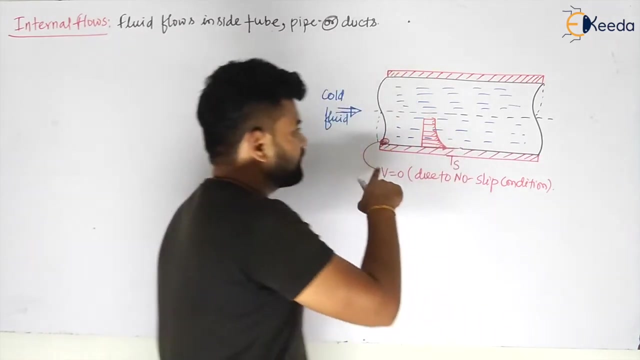 happen in this direction, my dear students, let us say, let us take it a small in this direction. what will happen in this direction, my dear students? the temperature will decrease like this, the temperature will decrease like this, and you will have a development of thermal boundary layer inside the pipe. my dear students, 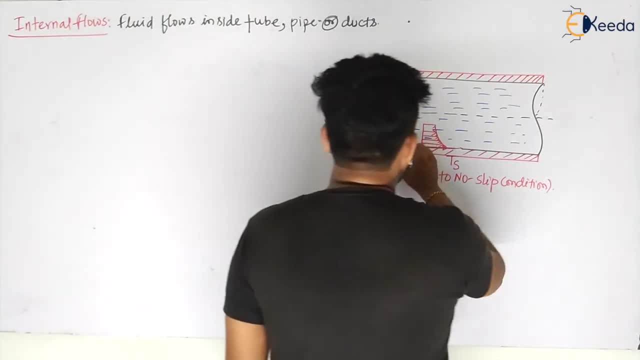 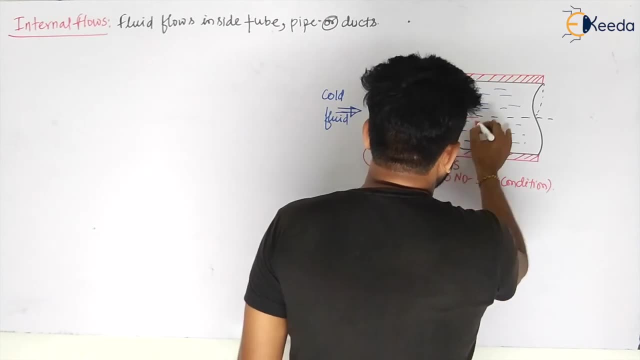 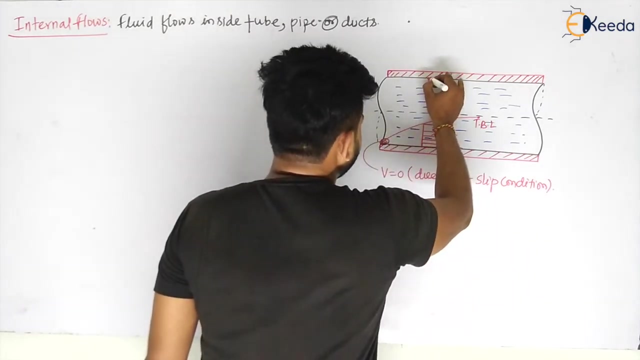 you will have a development of thermal boundary layer inside the pipe. how, so? like this. there will be development of thermal boundary layer, my dear students, thermal boundary layer. similarly, if you will see the upper side, my dear students, there will be again. the fluid flow will be like this. the fluid flow will be like this, my dear students, and. 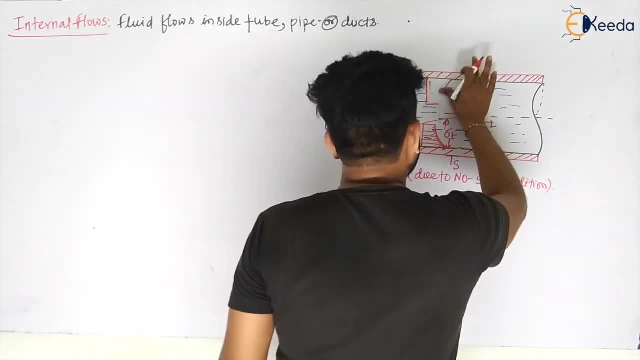 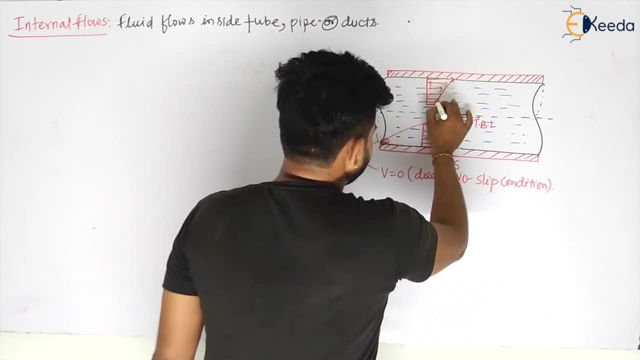 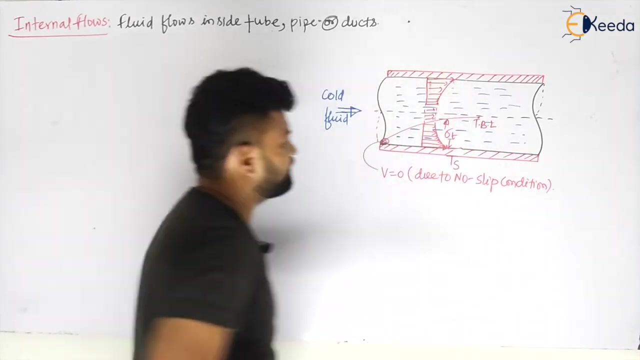 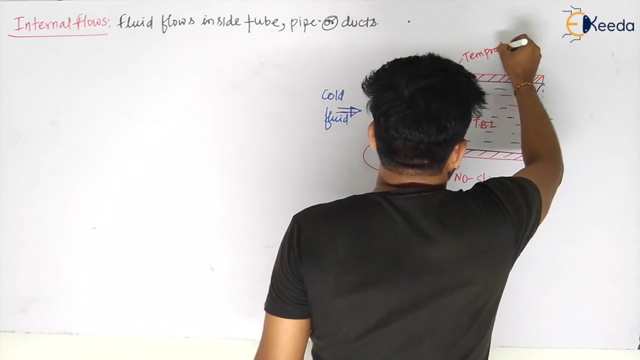 similarly, there will be, there will be development of boundary layer. yes, so this is the surface temperature and slowly, slowly, the temperature is decreasing and like this, like this, you will have a temperature profile. in this case, you will have a temperature profile. like this, you will have the temperature profilegt temperature profile. my dear, students. okay, so we have understood this concept. we have understood this concept like this: you will have the temperature profile, temperature profile enfim. that is what I would like to express this. another point in my above slide in our first class on cryptocom and 14 house more. this is one out there, remember. if you have any questions, you should not have answer this- call me. 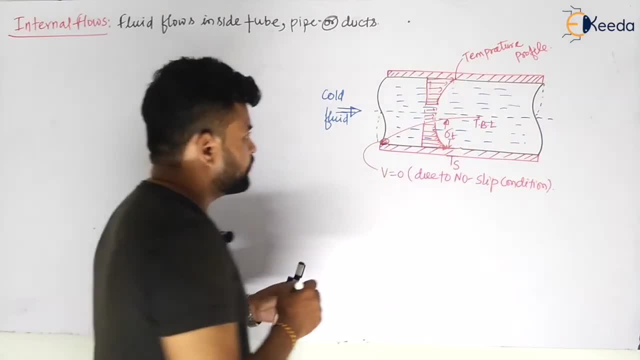 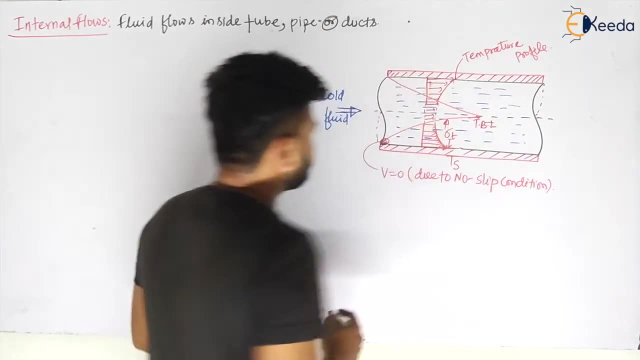 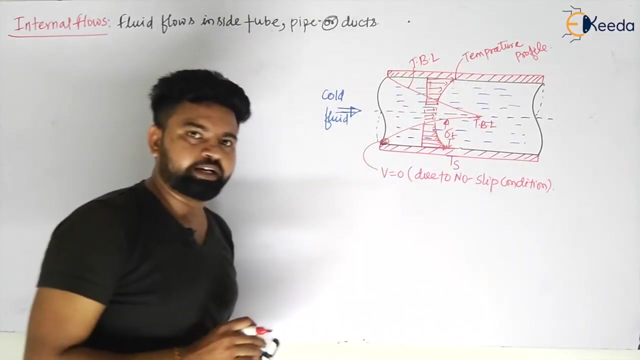 answer this. call me problem Aa. Now let us move on to the next concept. So, similarly, there will be some boundary layer development measurements. okay, Similarly, some TBL will be there, that is, thermal boundary layer measurements. thermal boundary layer. 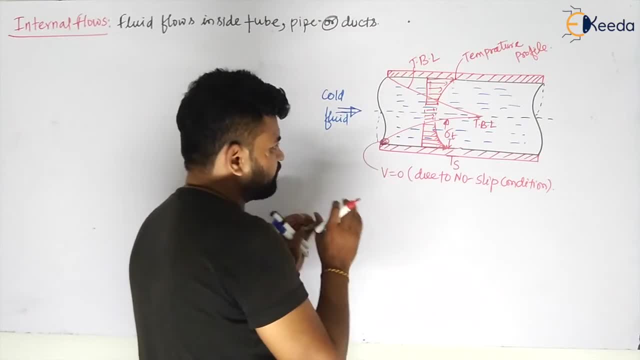 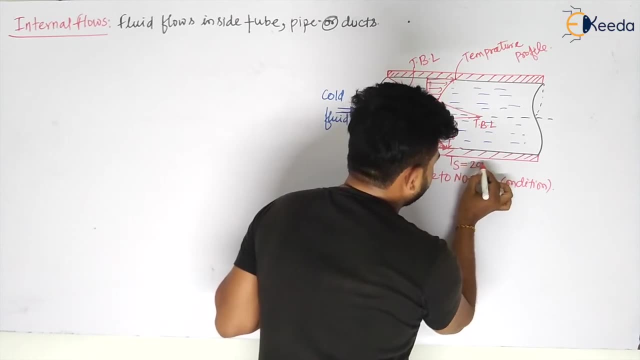 So if you will analyze a pipe or that surface heat transfer in the internal flows, what will happen? Let us take if temperature of this fluid surface, that pipe surface, is, let us say, 400 degree or 500 degree Celsius. 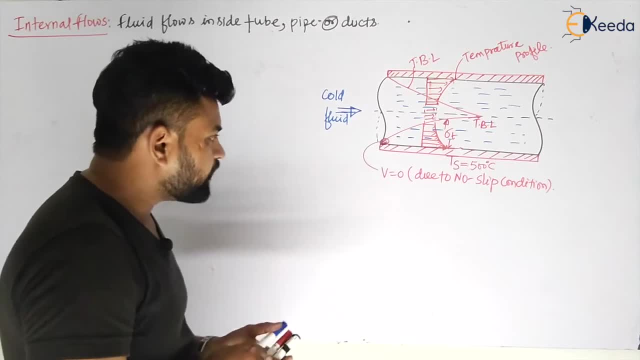 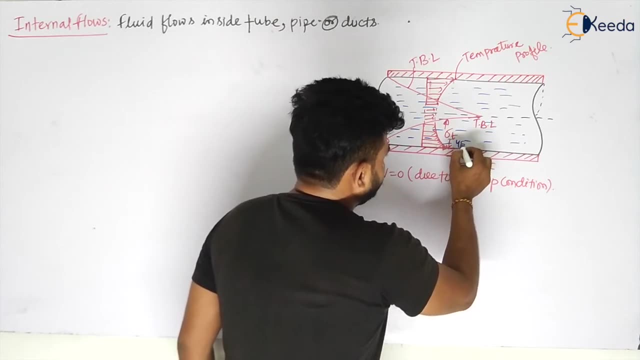 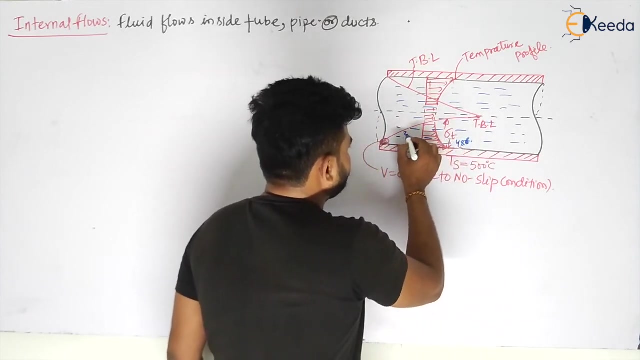 500 degree Celsius. So what is happening? Slowly, slowly, that temperature is decreasing. Let us say, here it is like 450 degree Celsius. or let us take it much closer, 480 degree Celsius. Then here it is like 340 degree Celsius. 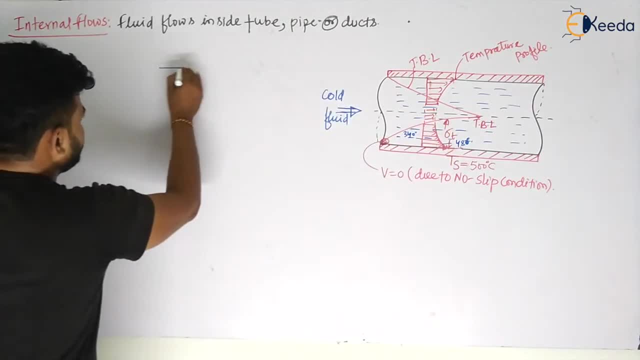 Let us take it like this, This side. So if this is your pipe, my dear students, if this is your pipe, what is happening? Let us see. If this is your pipe, slowly, slowly to the center, my dear students, the temperature is okay. sir, we have heard the concept now. 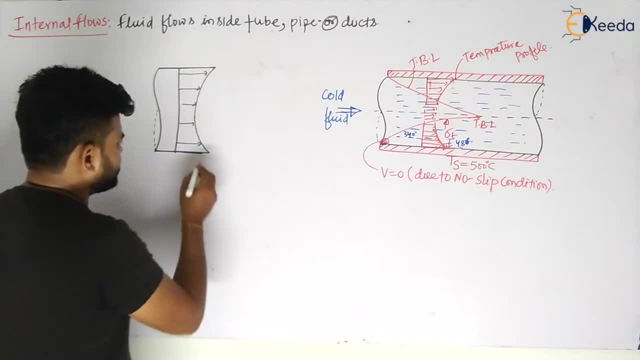 Now let us see. let us see If, my dear students, the temperature of this particular wall is particular wall, is, let us say, 500 degree Celsius I have taken, Then there the temperature is, let us say 450, then 350.. 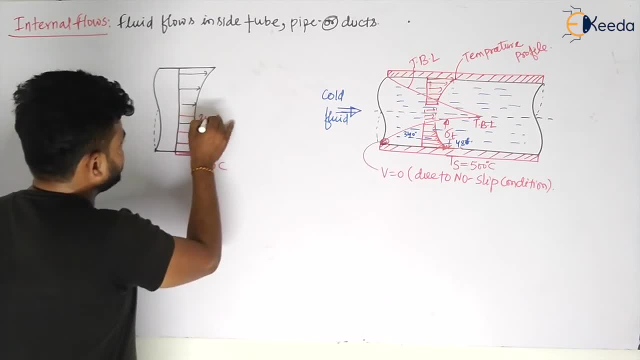 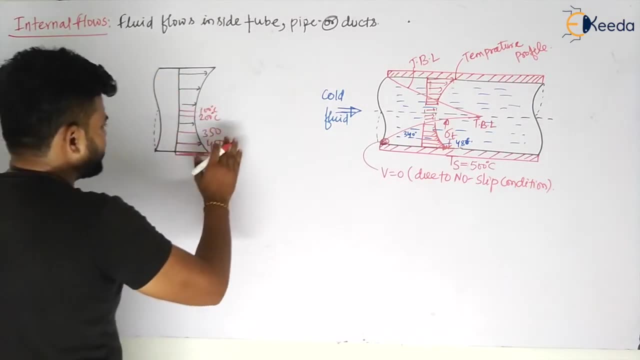 Then, then, then it is like 200 degree Celsius, my dear students, Then it is 100 degree Celsius, something like this. The temperature is dropping in this direction, my dear students, Or let us take it small. Let us take it small. 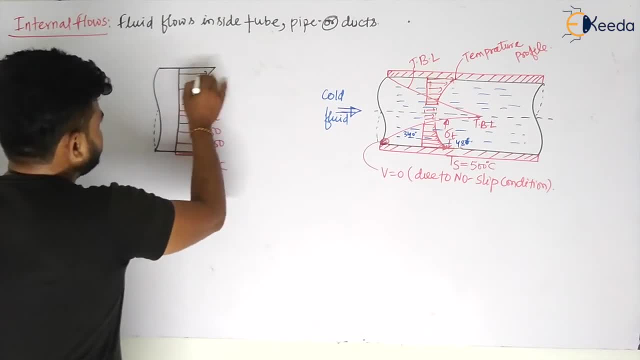 How about we can see. okay, Now if, similarly, in this case, also the temperature. if it is 500 degree Celsius, my dear students, then the temperature will decrease 480,, 450,, something like 350.. 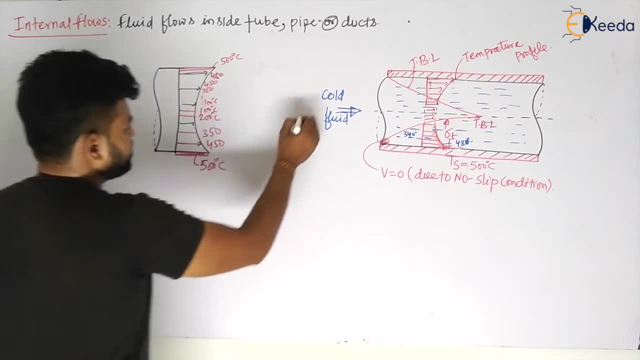 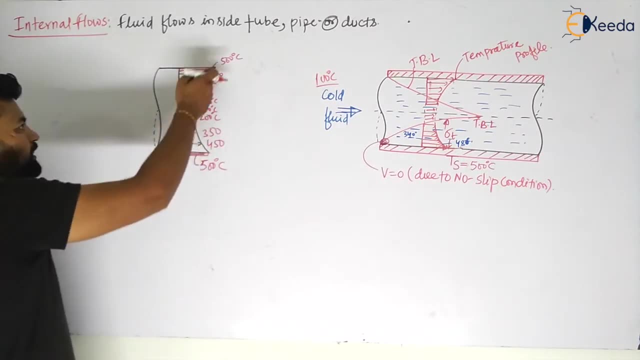 And then it will come to what 100 degree Celsius If this fluid is frozen, If this fluid is frozen at 100 degree Celsius, so slowly, slowly, the temperature is decreasing in this direction. Slowly, slowly, the temperature is decreasing in this direction. 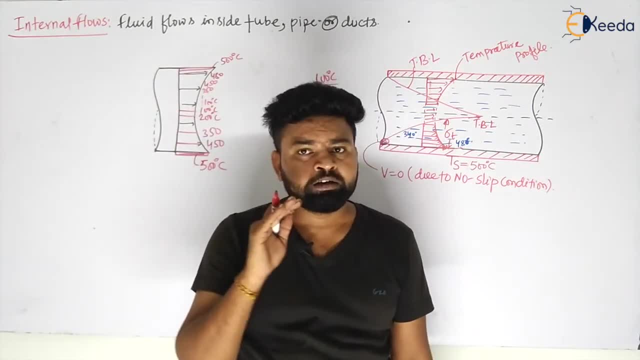 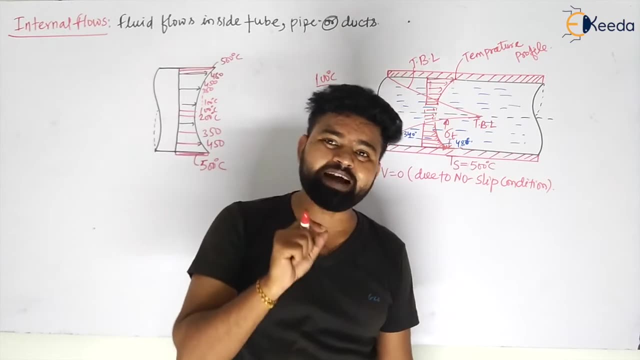 So we have to again like a like. we have taken a mean temperature at the fluid, like, at the flow over the surface of the plate, my dear students. Similarly, we have to consider a mean temperature. mean temperature in this case also. 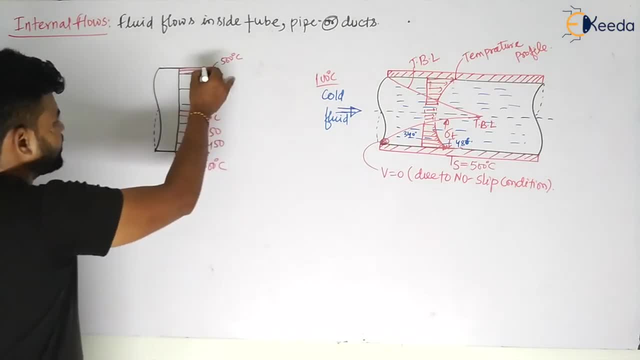 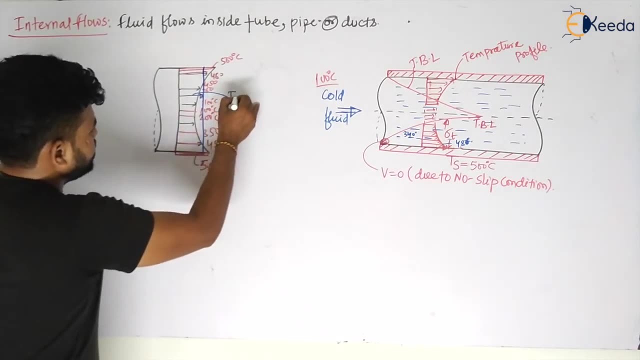 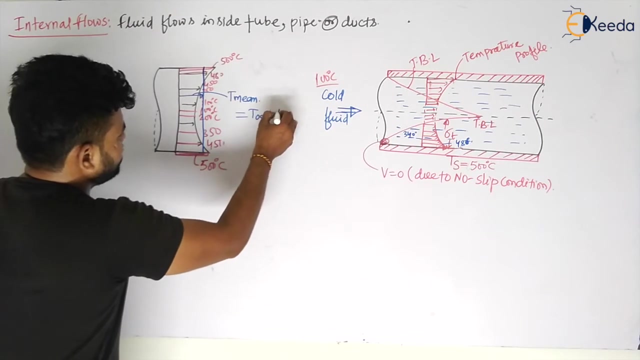 So how we will consider. So I will just take a mean temperature at this point, my dear students. I will take Tm, That is your T mean, my dear students, And I will take the average of both the temperatures, that is, fluid temperature plus surface temperature divided by 2.. 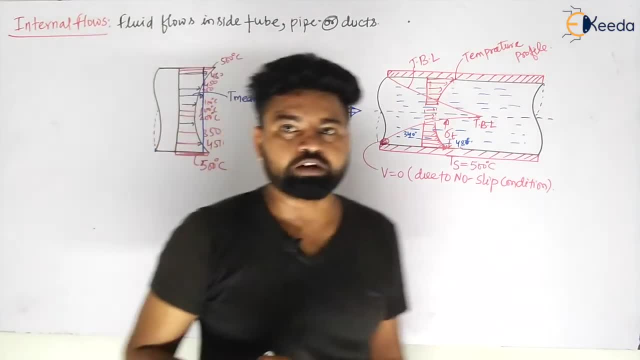 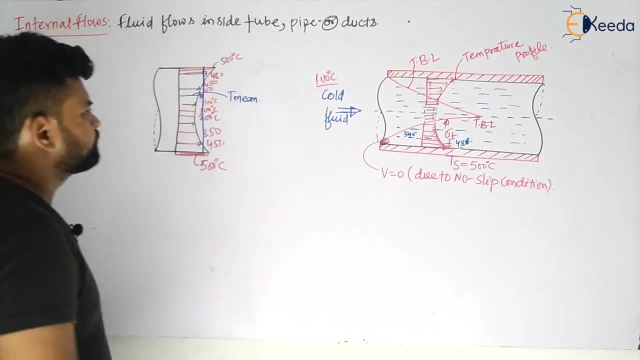 So we can, like this, can calculate the can calculate what We can calculate, like this: the mean temperature of the fluid. Let us fully analyze this. what is happening? Okay, Let us fully analyze it With the. now this is happening. 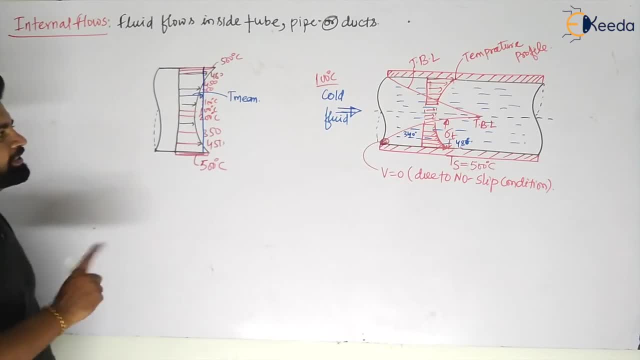 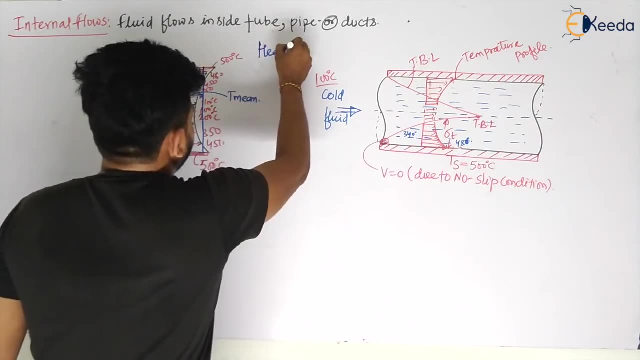 So if fluid is heated- fluid is heated or what- what is happening here? We are heating the fluid, We are heating the fluid, We are heating fluid, Heating fluid, my dear students. So if fluid is heated, what is happening? 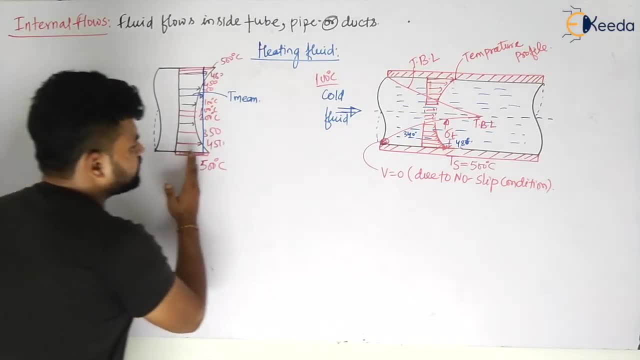 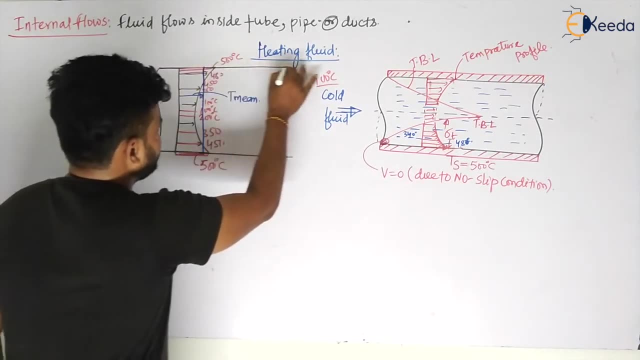 Slowly, slowly, the fluid is heating. Then, with the length of this length of this, my dear students, with this length of this pi length of this pi, my dear students, what will happen? Let us see So as that X. 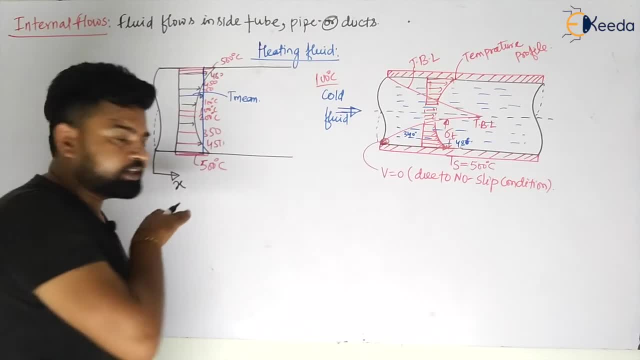 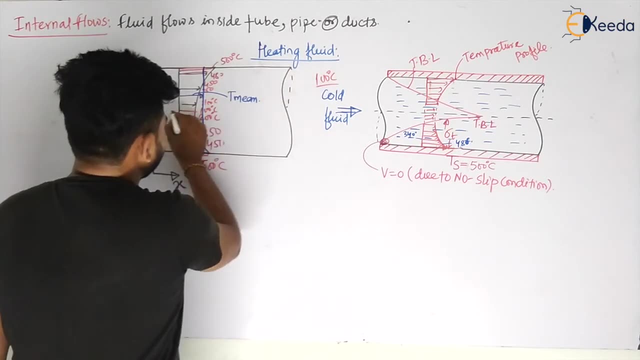 as that X increases in this direction. X increases in this direction, what will happen to the mean temperature? Let us see, my dear students, As X is increasing in this direction, my dear students, that fluid is continuously gaining heat from the surface. 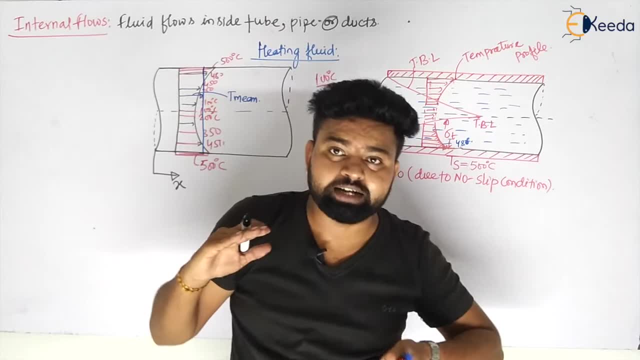 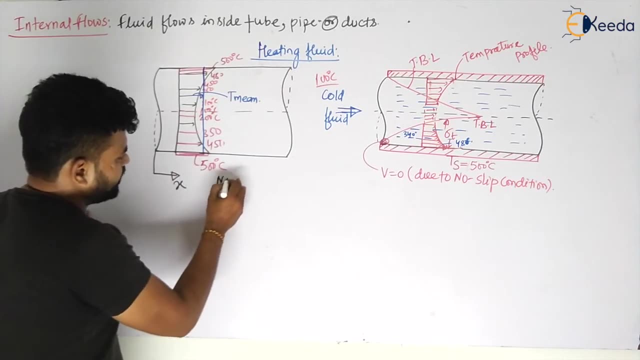 fluid is continuously gaining, gaining heat from the surface, and that mean temperature of the surface is increasing. Means of temperature of the surface is increasing As, so you can take a note here as as as fluid is continuously gaining heat, 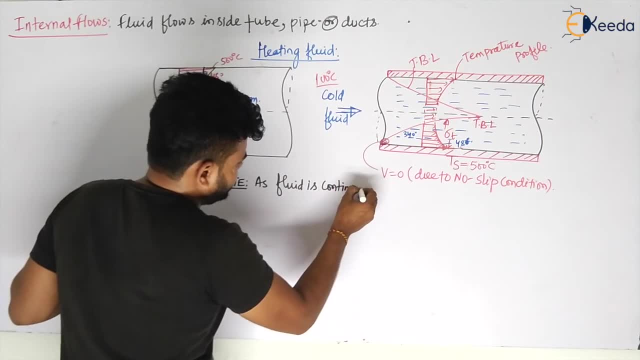 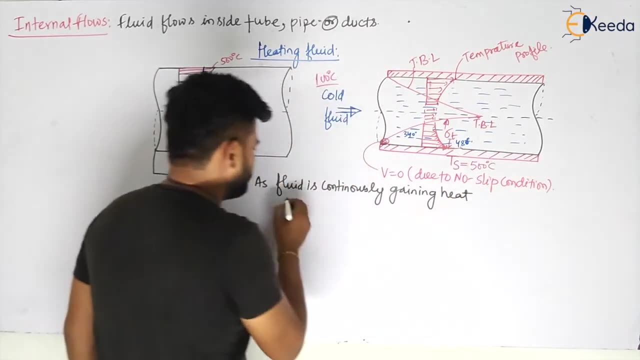 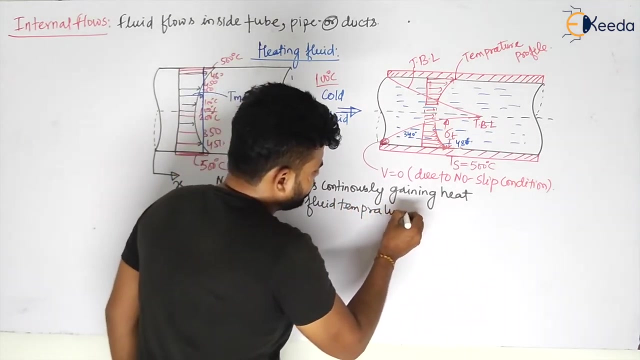 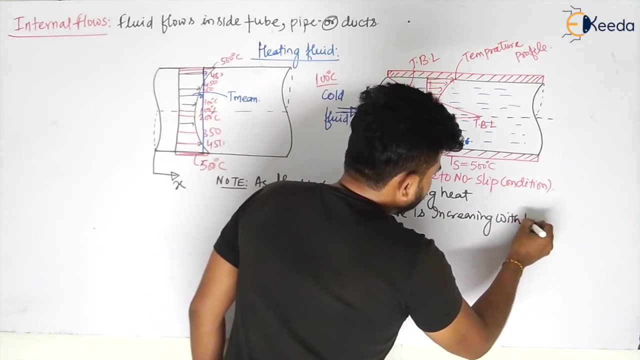 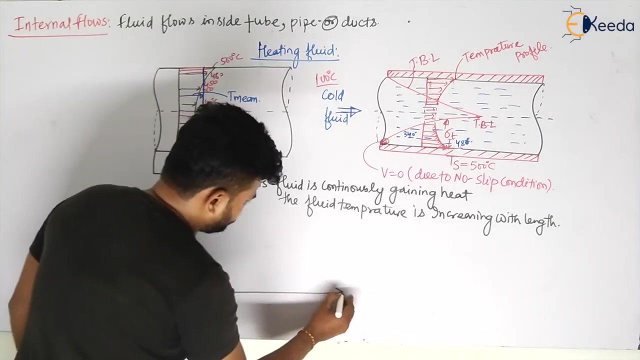 fluid is continuously gaining heat. the fluid temperature is increasing. fluid temperature is increasing, is increasing with length, Yes or no, my dear students? Yes, sir, Now this temperature is increasing, my dear students, That fluid temperature is increasing in this direction. 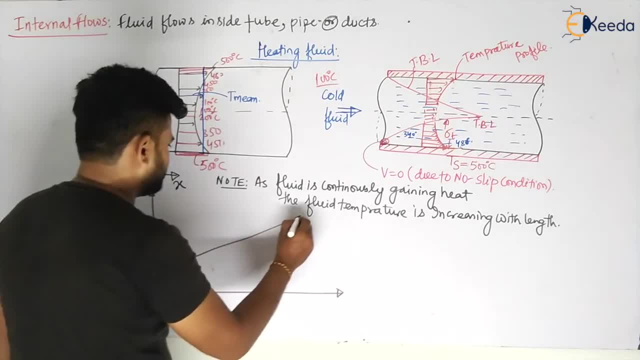 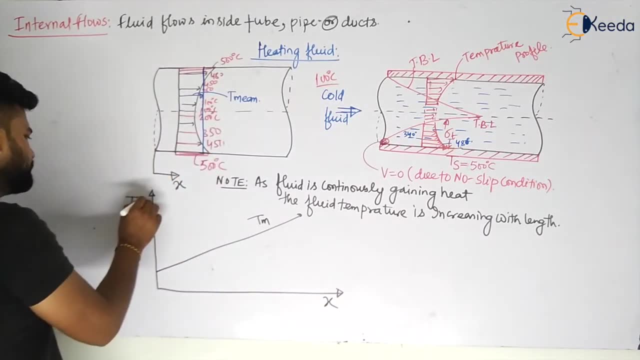 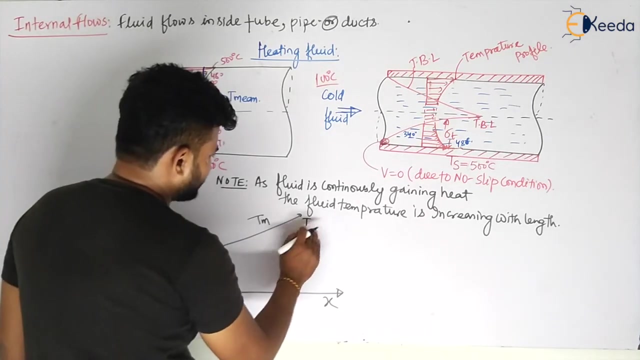 Yes, Sir, the fluid temperature is increasing like this. Let us say: this is your Tm, along X, Along X. T is the fluid temperature, T is the fluid temperature. So from here inlet to, that is, from inlet to exit, exit. 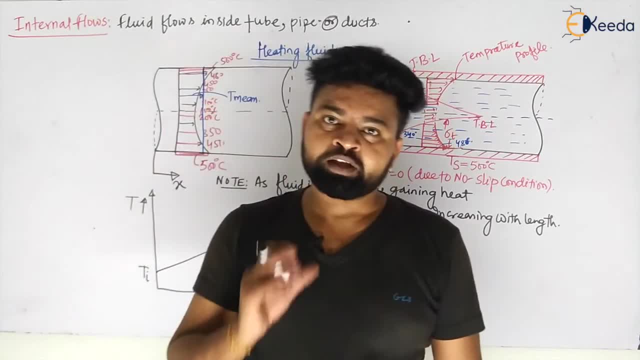 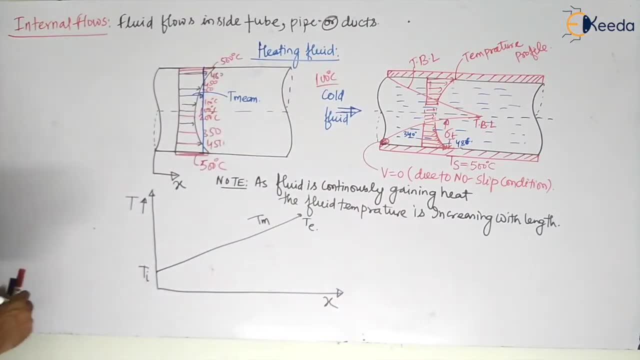 your fluid temperature is increasing slowly, slowly. Okay, So there can be only two cases: One is heating and one is cooling. So cooling of fluid will be done. A cooling of fluid will be done. What will happen? Let us analyze it completely. 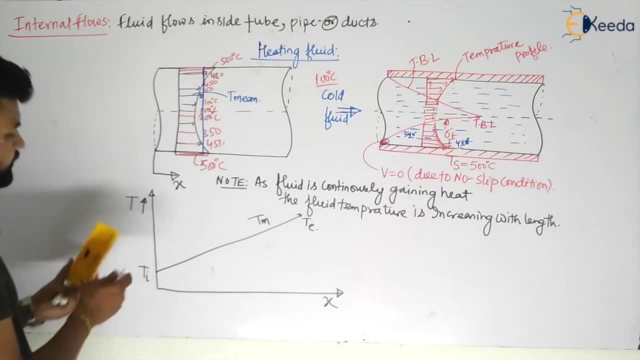 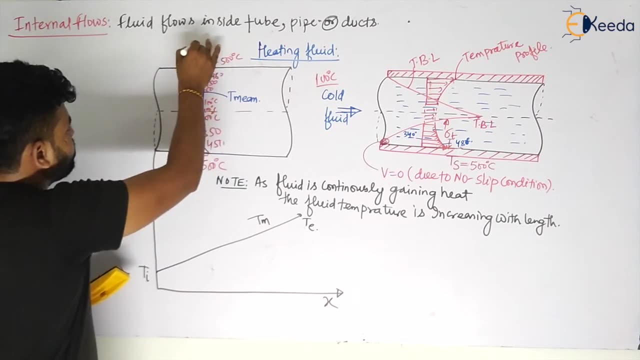 So a cooling of the fluid will be done. So that is your T mean, And T mean how much We have to tell them this. So this will be your T mean, my dear friends. Okay, So now, a cooling of the fluid will be done. 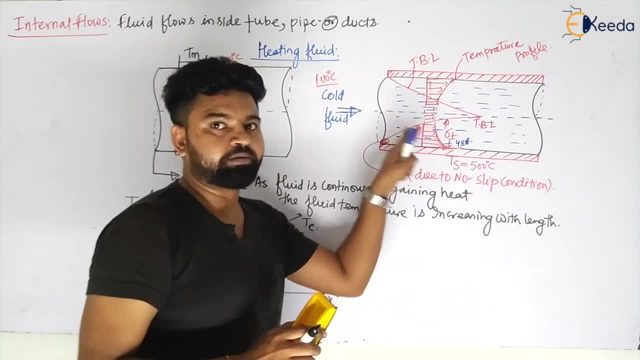 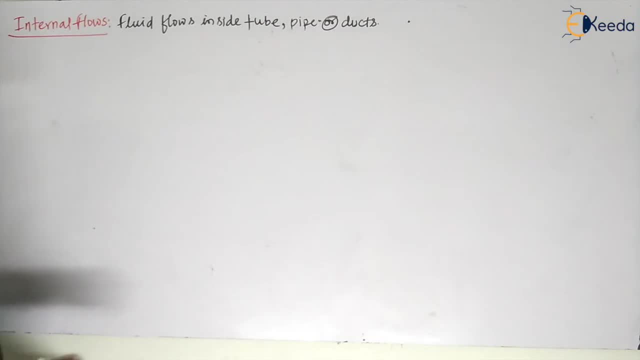 What will be there layer and how the thermal boundary layer will be developed. let us see. so if i am just cooling the fluid, i am just cooling the fluid, my students, what will happen? let us see. let us see the case. second, cooling of fluid. cooling of fluid, my students. so now the temperature of the fluid, that is t. 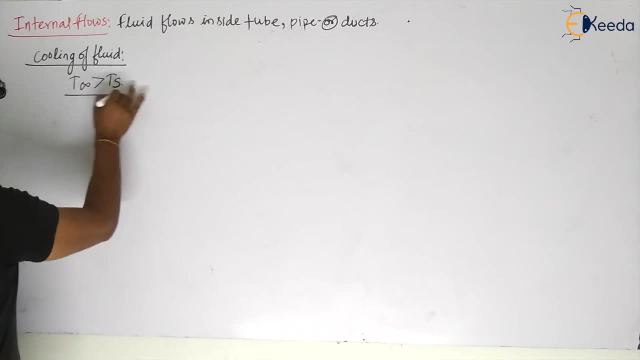 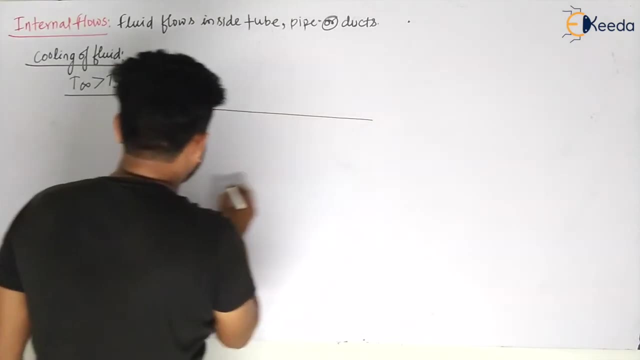 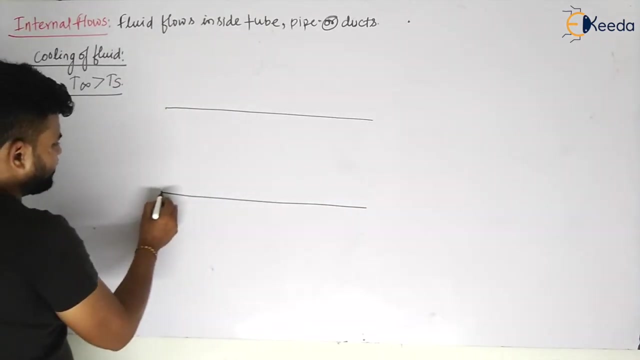 infinite is greater than t surface. t infinite is greater than t surface. my students, and this is your pipe, let us analyze all the concepts of fluid mechanics also, so that you will not have any problem. so let us say: the fluid is entering inside this from here, from some like: this is your. 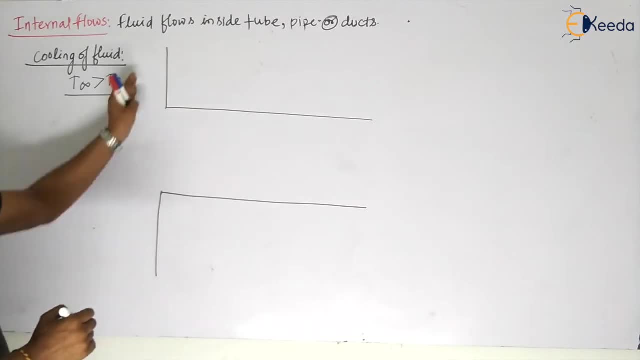 large, this is your large carrier and fluid is flowing like this. so fluid is flowing like this. this is your fluid. so slowly, slowly, what will happen? first of all, in this pipe, my students, in this pipe, the fluid will come inside this, fluid will come inside this. so what will happen when fluid will come this side? 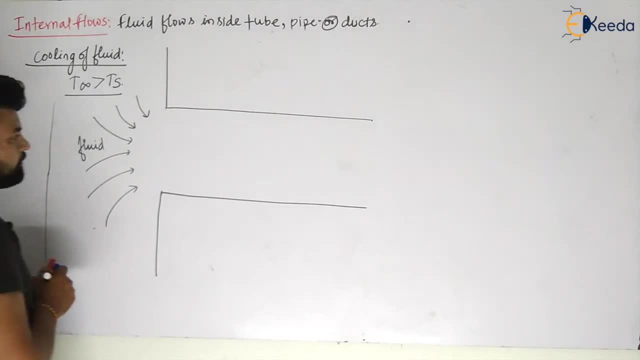 then there will be some water, like we are taking the cold fluid now, or cooling of fluid we are doing, then the fluid will be hot. this will be a hot fluid. so first of all, this will increase, this will come, and if i will talk about the fluid mechanics little bit, let 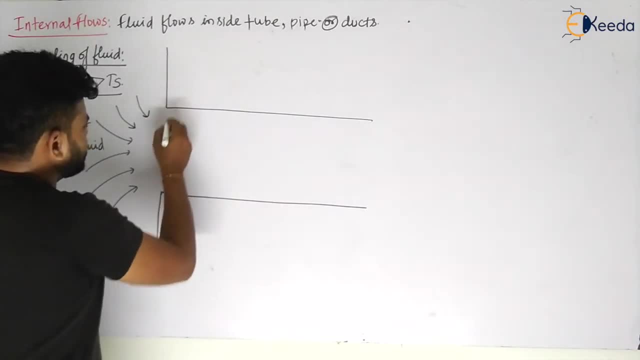 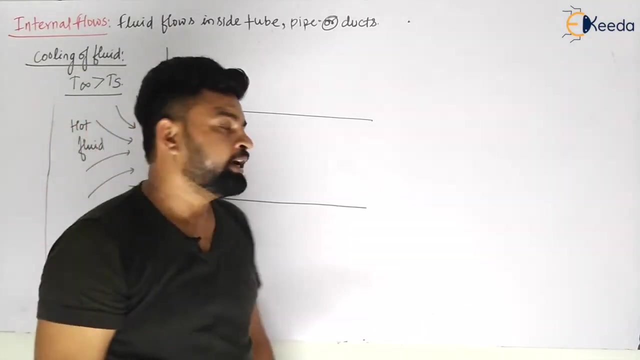 us touch that part so that you will be able to understand all the questions. now, as the fluid is coming in this direction, then some velocity, if you will see, some velocity is like, continuously like this. the velocity will be continuously like this, my dear students, and slowly, slowly, slowly, slowly. 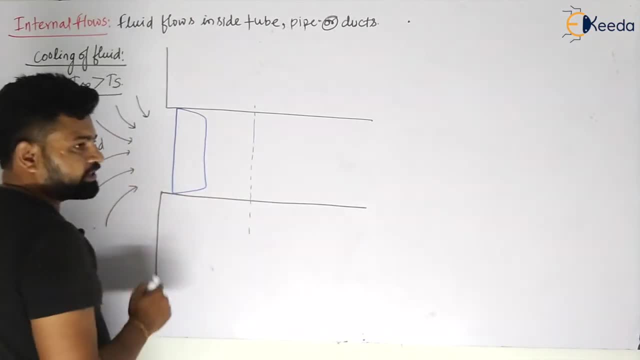 after some length of the pipe, after some length of the pipe, the fluid will come inside this pipe. what will happen? slowly? slowly it is coming from the carrier and slowly it is entering here, my dear students, and let us say: this is your velocity profile. this is your velocity profile. maybe you 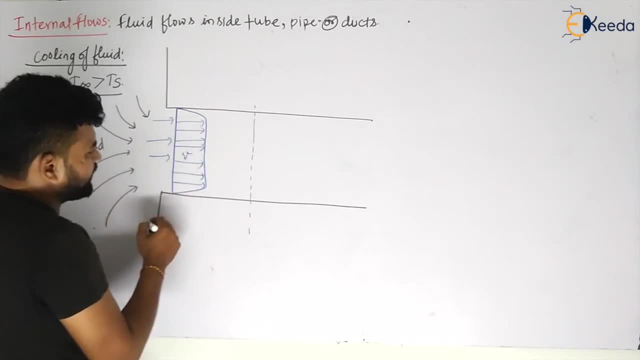 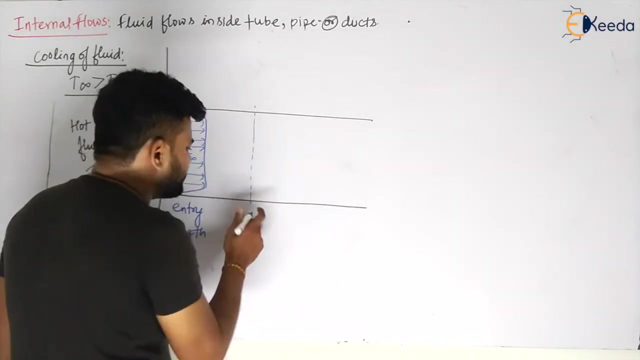 have gone in this topic or you have studied this in your fluid mechanics. so if fluid is moving with this, like this, so after some time, after some length or entry length, my dear students, entry length, we call this entry length- what will happen? the fluid will be fully developed and the fluid will be. 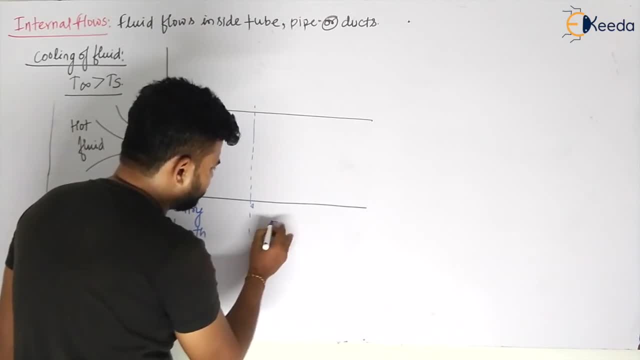 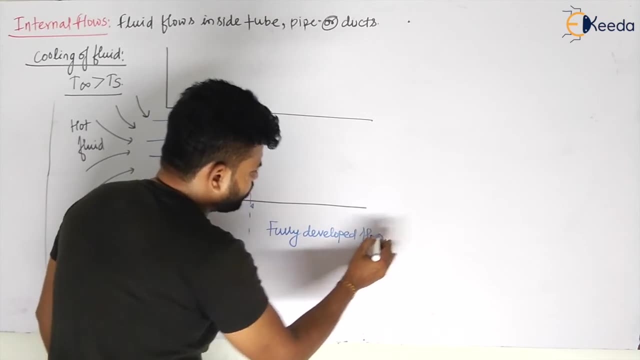 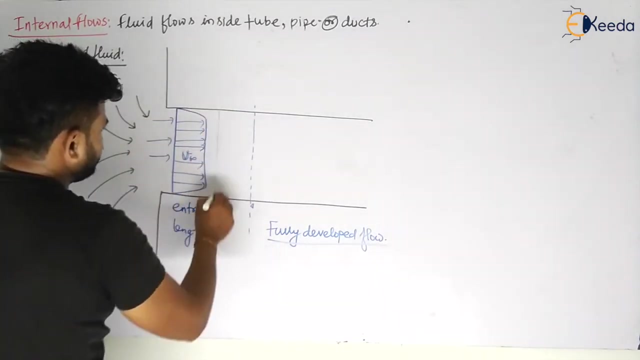 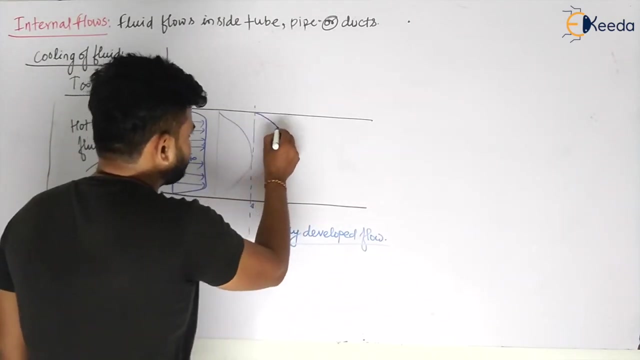 fluid will be, or we can call it like fully developed flow. fully developed flow, developed flow, when the velocity profile will become continuously. now, slowly, slowly, that velocity profile will change. slowly, slowly, that velocity profile will change and after some length, this velocity profile will become constant, my dear students. this velocity profile will become 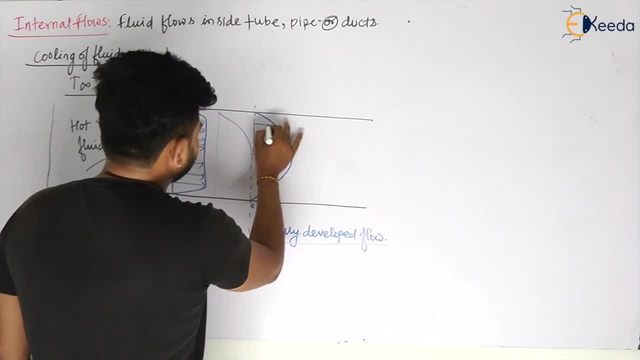 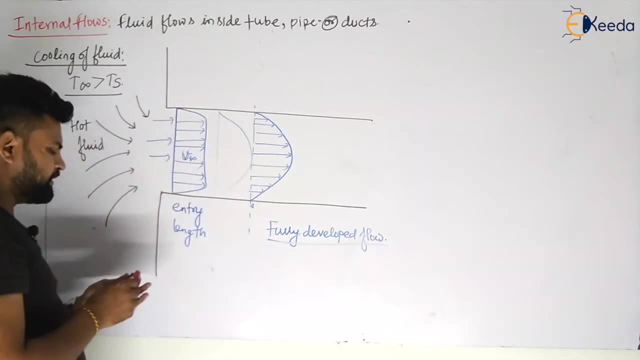 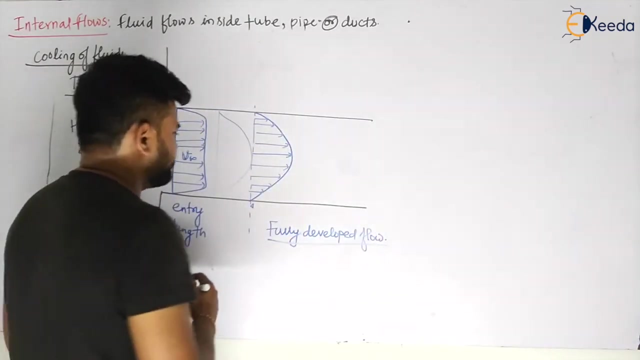 constant like this and why it is happening. let us analyze it. if you have not felt the concept, let me explain this also. so what is happening, my dear students? again the same concept: when fluid have entered, this fluid have entered and that has become the fully developed flow. now, what will happen? the molecule? 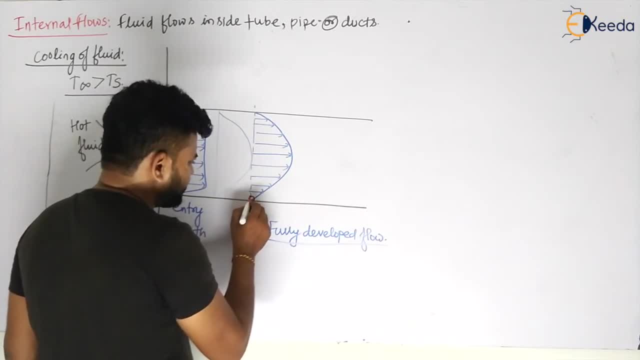 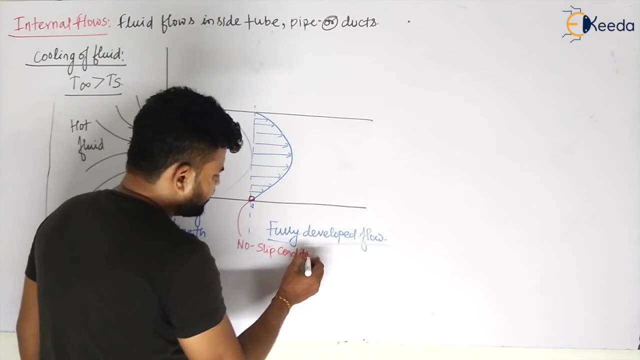 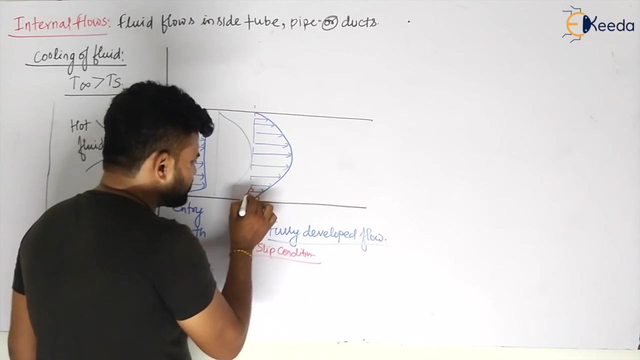 of this particular fluid will come to this position, my dear students, and it will felt the again no slick condition, no slick condition and due to which this will come in rest. this will come in this and continuously this layer will come in rest and again the layer which is upon this. 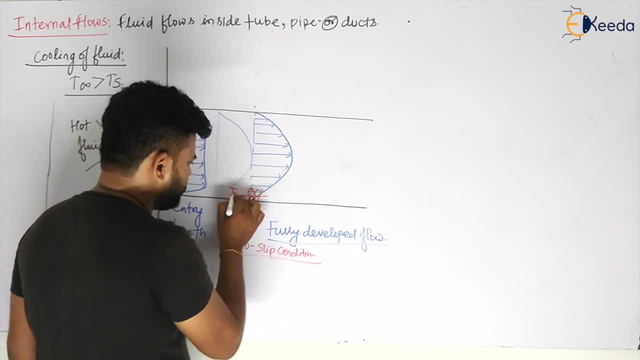 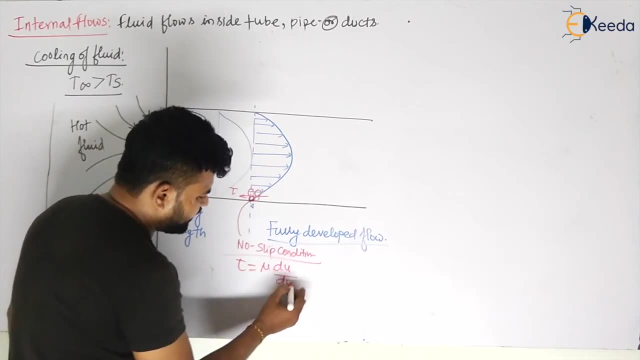 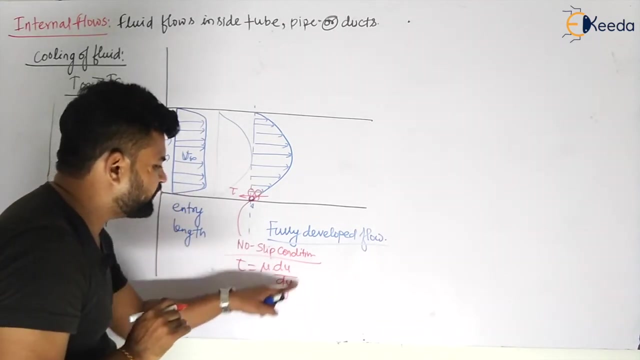 my dear students, it will felt some tau, my dear students, tau some shear stress, and shear stress because of what tau you know: mu del u by del x, my dear del u by del y. my dear students, if i will take that y in this direction, okay, and slowly, slowly, what will happen? due to shear stress, due to that, 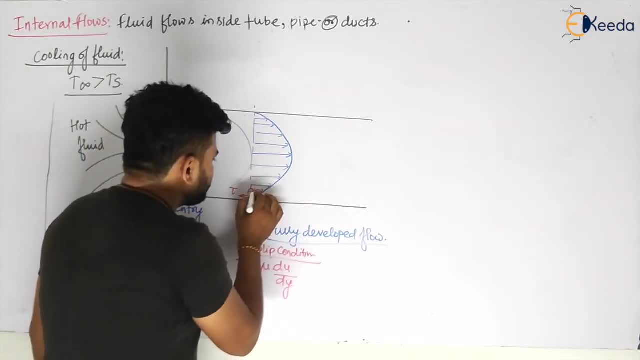 surface resistance. what will happen? the velocity will this? this rest, that fluid layer which is at rest will try to just slow down that through for time, sudden that you and similarly the velocity of this layer will decrease, this layer will decrease and again this layer will like: if this is going in this direction, this: 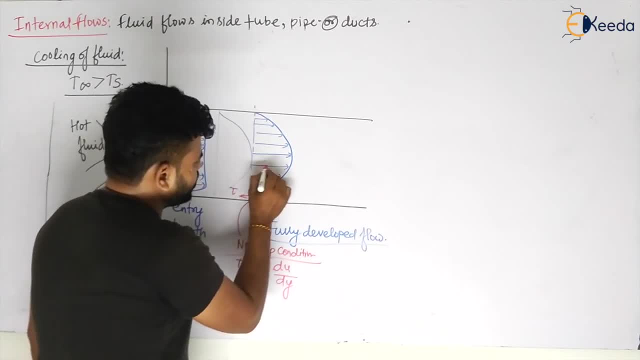 layer will put a shear stress in this direction. if this is going in this direction, this layer will like lower level, will put a shear stress in this direction. so, like this, what will happen? the velocity will decrease up to this level. Quark channel of this Diesel 정도. the video: 14 lot in 2ji Quark channel, in 2D station, the butsea level out because six buttons as a Pika, letters are whichever, and then if you cut out A Ayurvedic commons, either arrow, you will get Felêtre beau. so in this situation mean, if your inner shaft is not the output, all. 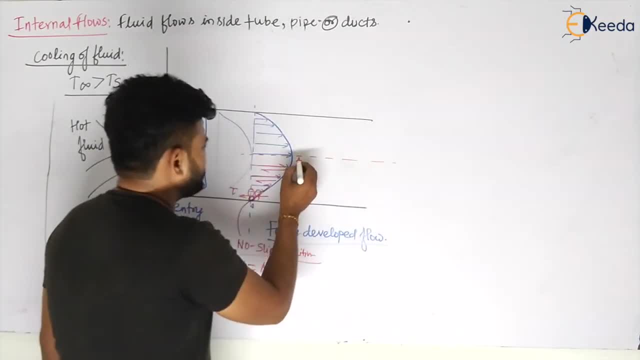 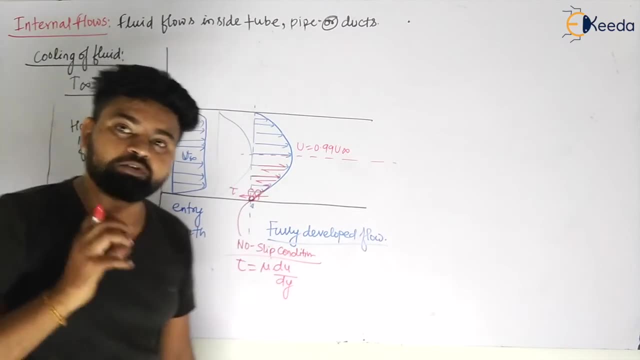 this, but at the center, my dear students, the velocity will become equal to. how much? that will become equal to? u is equal to 0.99, u. infinite, my dear students. like that, the velocity profile will be developed in this. okay, now, if you will talk about the hydrodynamic boundary layer, 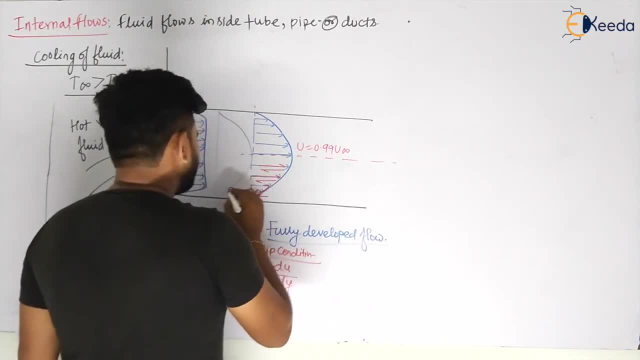 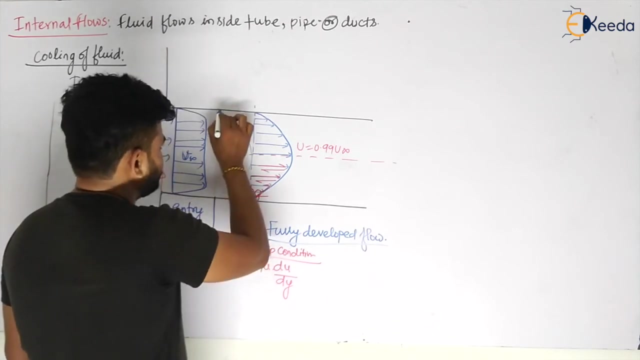 so what will happen? so, if you will talk about hydrodynamic boundary layer, the hydrodynamic boundary layer will be developed, something like this. i have analyzed this like this: so, uh, from here the uh. this must be something like: let us take this here. let us assume that there is. 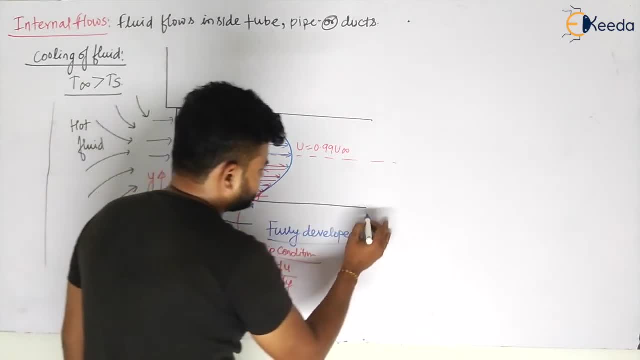 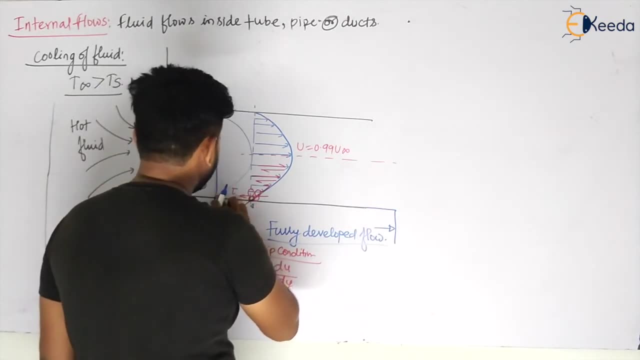 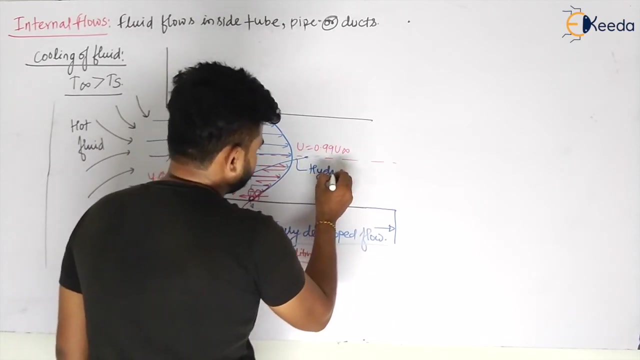 let us assume: okay, now i'm taking, because i have shown you this here. so what will happen? this will be something. this will be something like this, my dear students. this will be something like this. so this will be your hydrodynamic or hbl. let us try to take hbl where hbl is equal to. 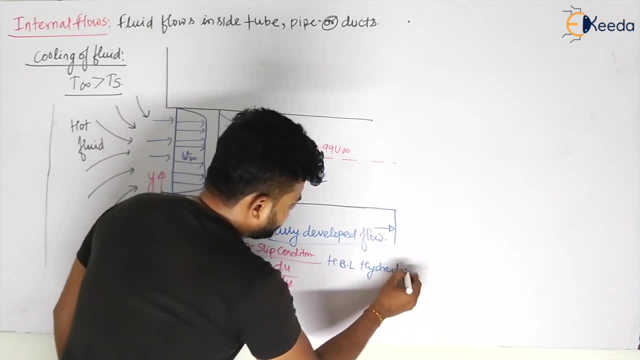 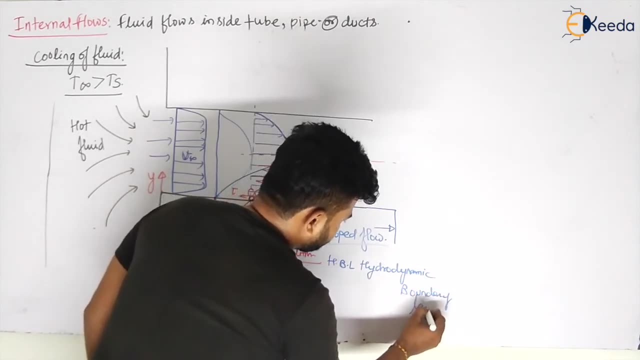 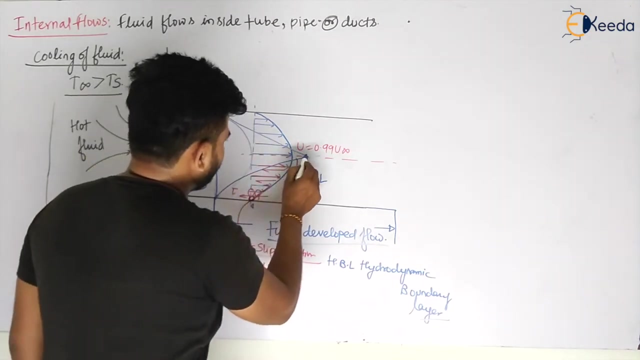 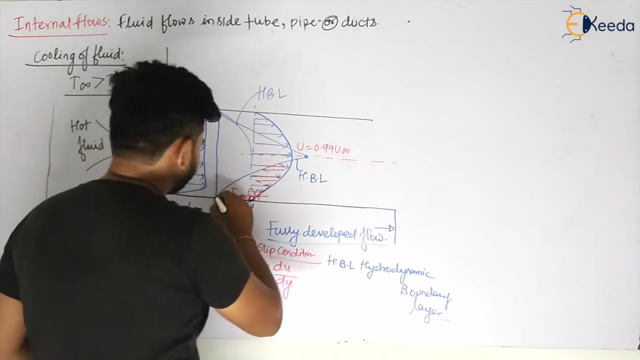 hydrodynamic, hydrodynamic boundary layer, boundary boundary layer, yes or no? so, similarly, again from this point of view also, there will be some development of hydrodynamic boundary layer. that will be development hbl. my dear students, hbl, if it is not clear, let me take the another color. so this will be your hbl, like this: 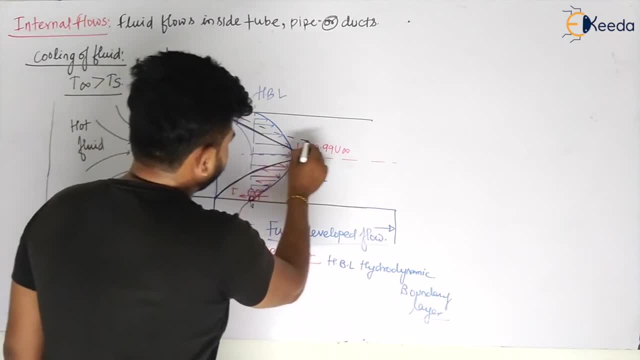 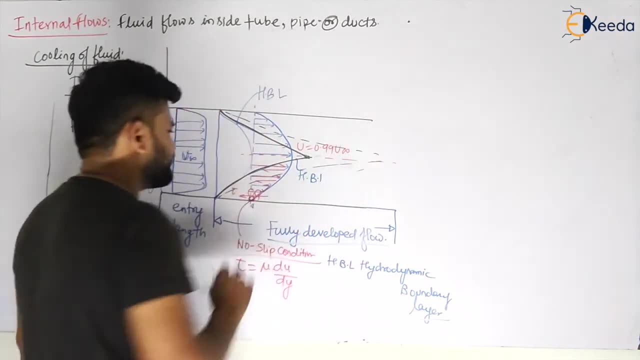 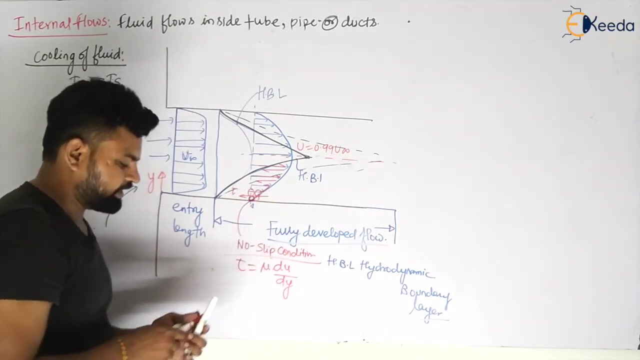 and similarly. these will develop like this. so there will be development hydrodynamic boundary layers continuously like this, continuously like this, my dear students. okay, now let us talk about the thermal boundary layer. that is your hot fluid, my dear students. now the surface is cold. let us extend it. let us extend it so, if you will see the thermal boundary, 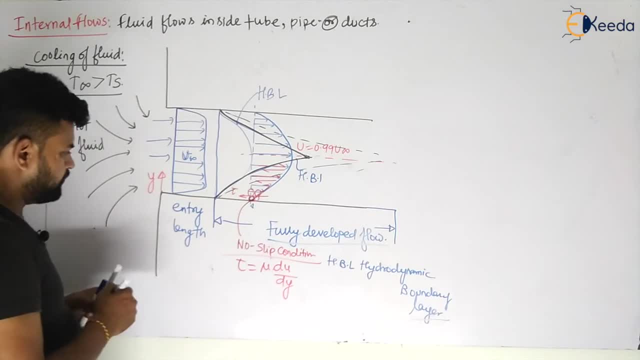 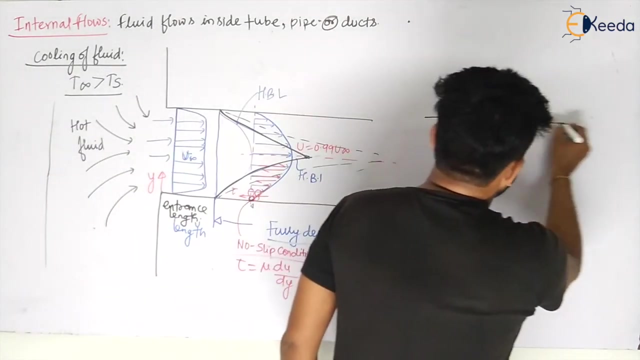 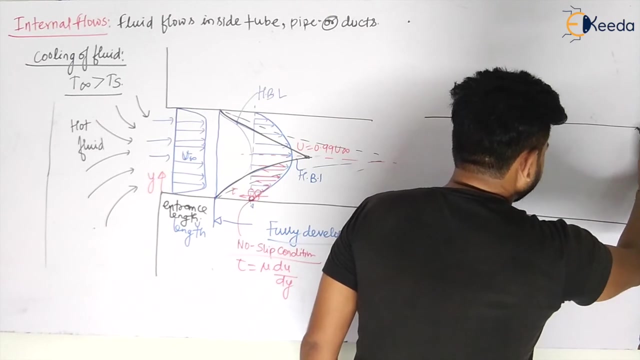 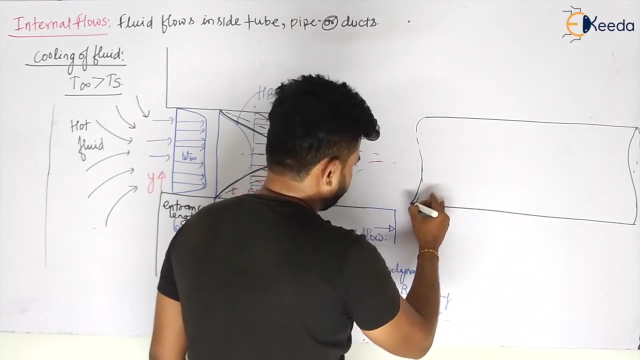 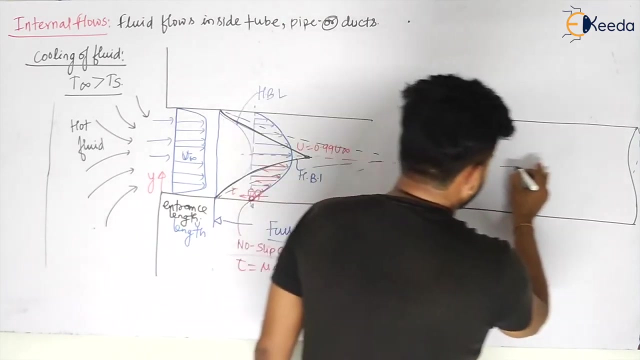 layer will be something that is called your entrance length. and this length, my dear students, let us analyze also if this is something like this: again, the cold fluid is flowing inside this pipe. let us see, the cold fluid is flowing inside the pipe. okay, so when cold fluid will do inside the pipe or will come inside the pipe, let us say this: 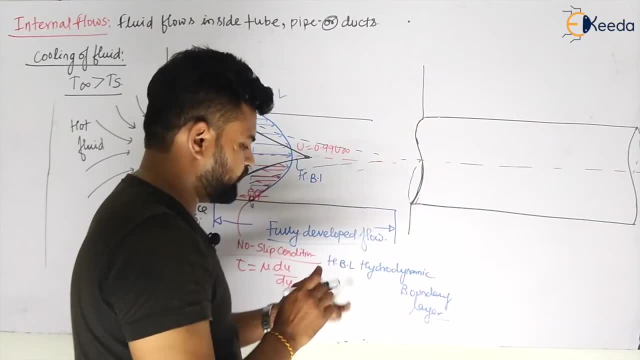 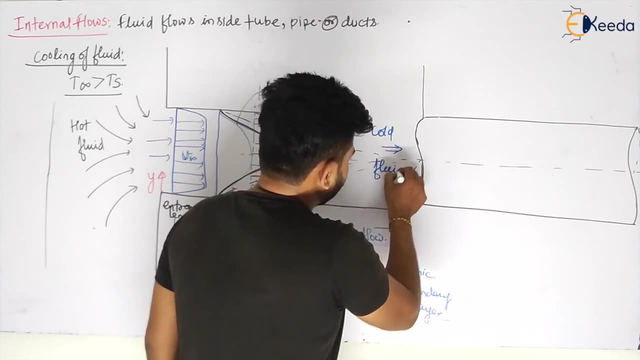 is your some carrier which is carrying the fluid in this direction, my dear students. so what will happen like cold fluid is coming in this direction? cold fluid is coming, okay. so when cold fluid is coming in this direction, it will flow inside the pipe, yes or no? yes, 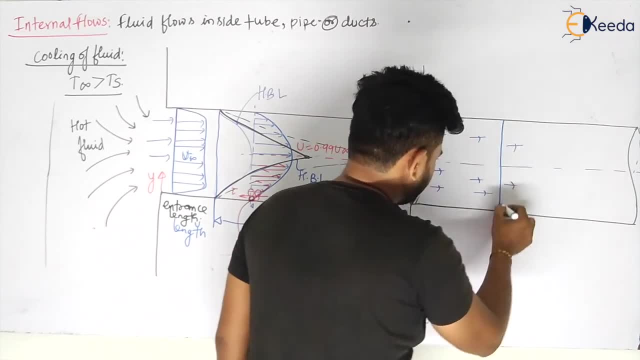 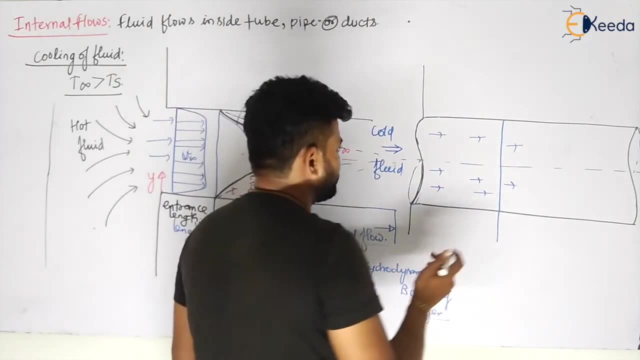 sir, it will flow inside the pipe, but after some length, after some length of the pipe, this will be like thermal boundary layer will be there. so this is, the thermal boundary layer will be fully developed. thermal boundary layer will be fully developed. like before, it is like this. before, it is something like this, my dear students, something like this then, 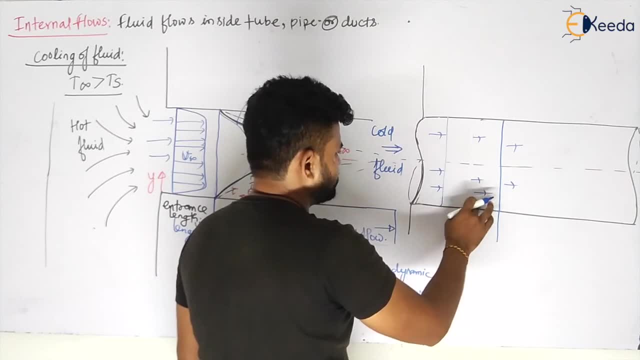 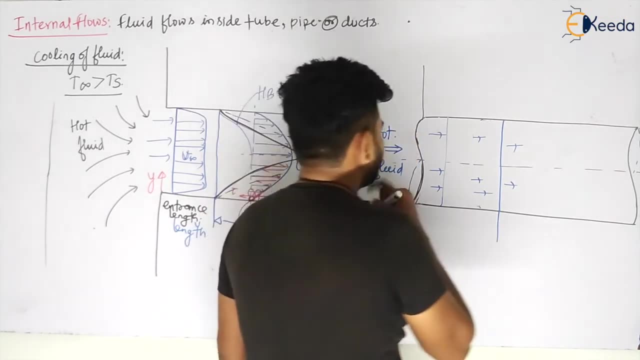 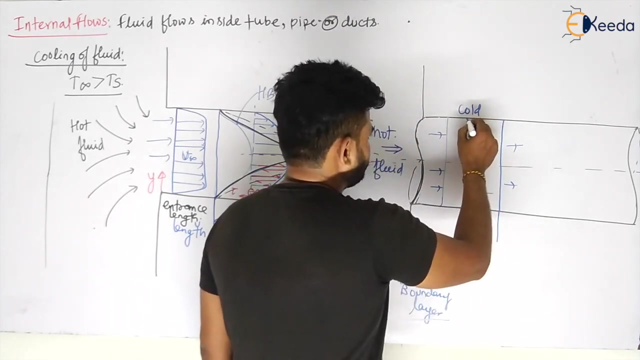 it is becoming like fully developed. or let us take, because this is now: your fluid is hot, fluid is hot, hot fluid we are talking about because cold we have discussed, so the fluid is hot and plate is cold, so the temperature will decrease. so this will be something like: 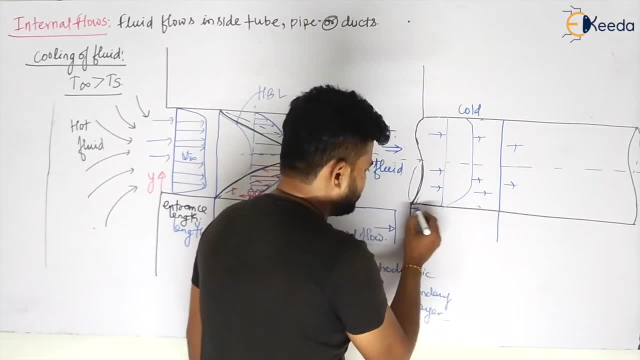 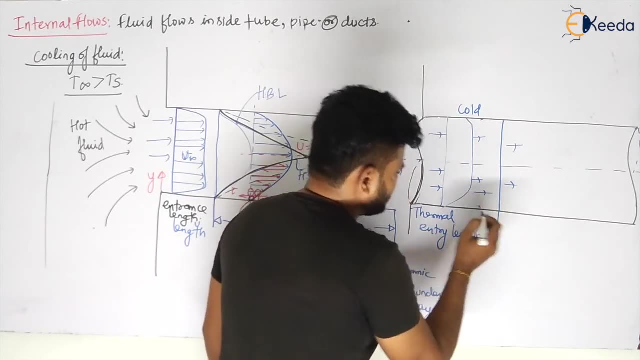 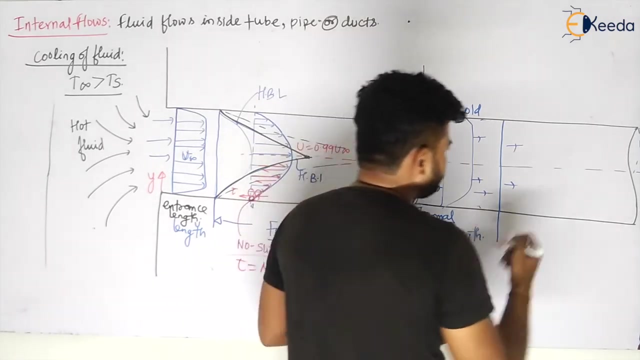 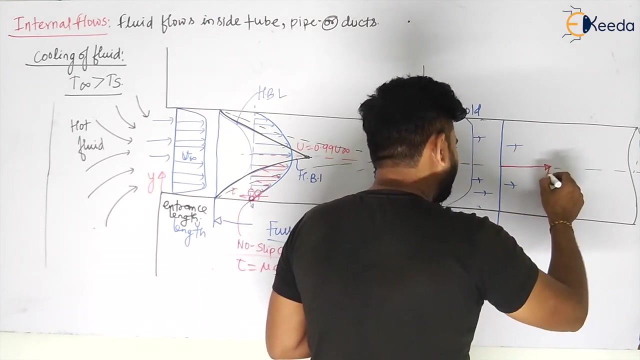 this. so, after this thermal entry length, thermal entry length, my dear students, what will happen? the thermal boundary layer will be fully developed. fully developed how? let us see so now, in this case, my dear students, the fluid is hot, which is having high temperature, and slowly, slowly, what will happen? the temperature of fluid will decrease. like this, my dear students, temperature. 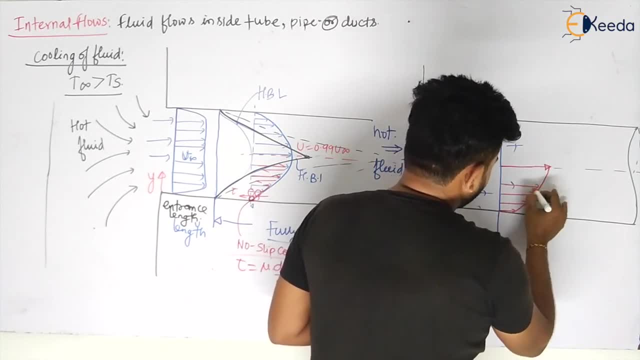 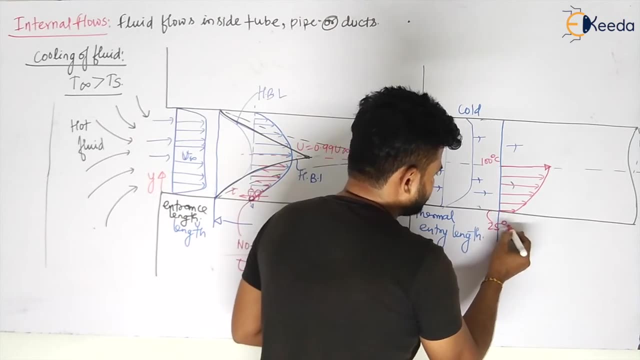 of fluid will decrease like this. so if you will take, let us see, the fluid is at 100 degree Celsius and that is at 25 degree celsius. so slowly, slowly, what is happen? so the fluid will transfer heat to the adjacent layer and temperature of this will decrease. 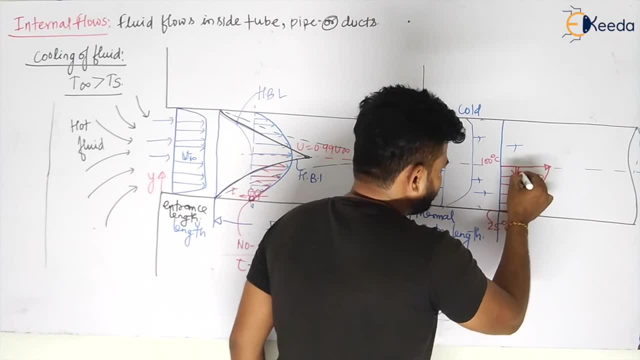 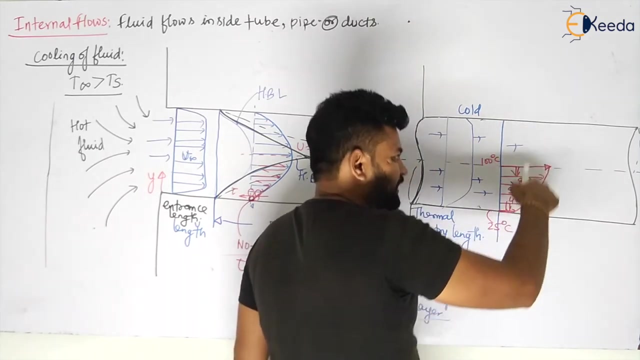 let us say 80 degree Celsius, or let us say from here 25 degree Celsius. now we transfer heat, it will come like at 40 degree Celsius, then 30, 50 degree Celsius. so, like this, temperature will decrease in this direction when you are cooling the fluid measurements and the temperature will decrease in the direction. 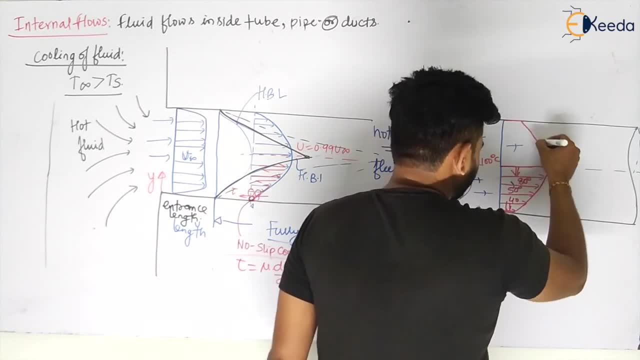 when you are cooling the fluid measurements and say that this is more or less the same other side which we have to think will stop and let us see the Next abundance decades now, like this, there will be your, there will be your development of what? the development of your thermal boundary layer, my dear students, development of. 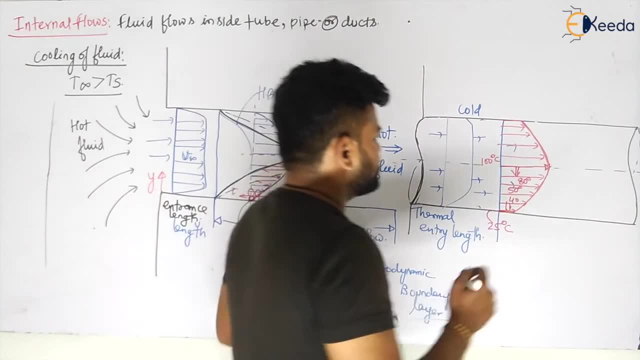 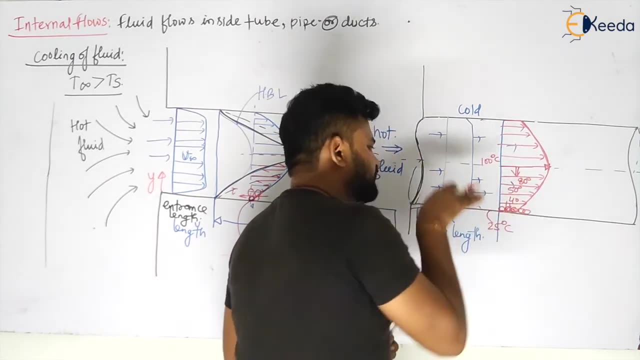 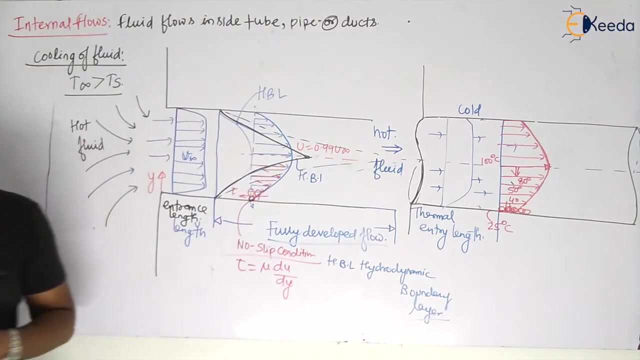 thermal boundary layer like this- okay, now this is called your what. so like this: when fluid will touch this surface, you do not sleep condition. what will happen? this will come to rest. then again, the heat transfer. you have seen this concept. let us see what will be the. let us see what will be the thermal boundary. 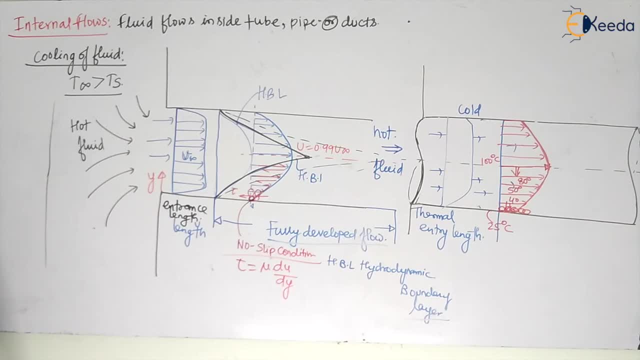 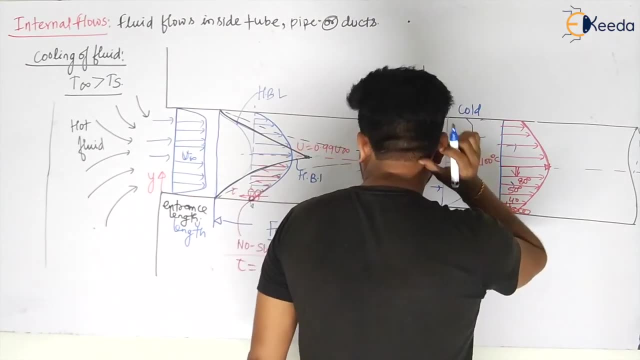 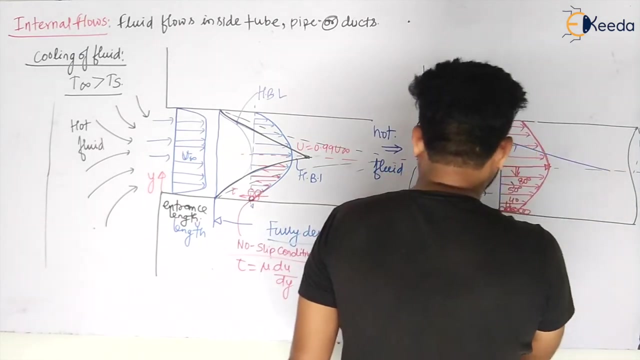 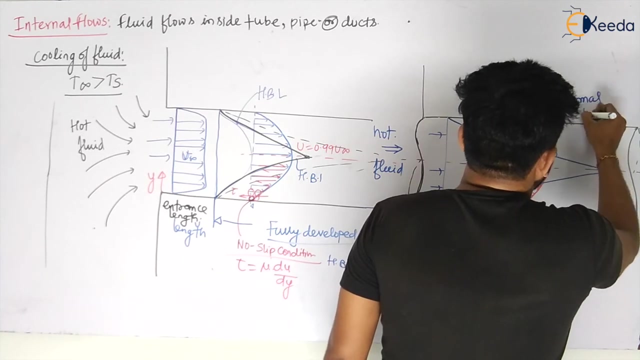 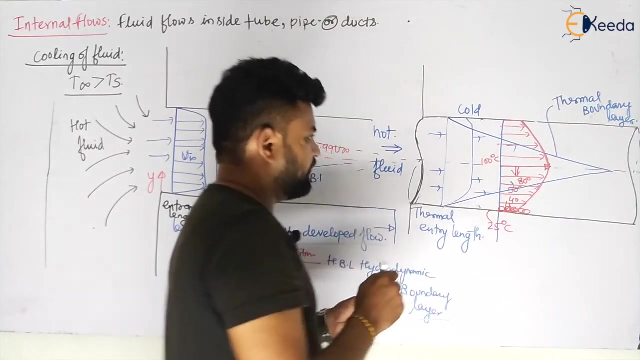 layer, my dear friends, what will be the thermal boundary layer? so the thermal boundary layer will be like this. let us see so from here. if I will take the thermal boundary layer will be something like this. that is your thermal boundary layer. okay, my dear students, and in approximation to this, if you will see the hydrodynamic boundary layer, it 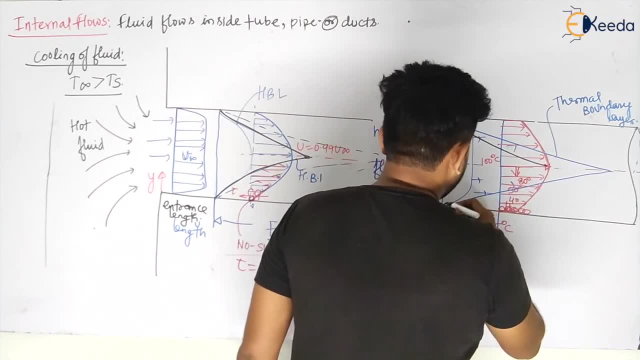 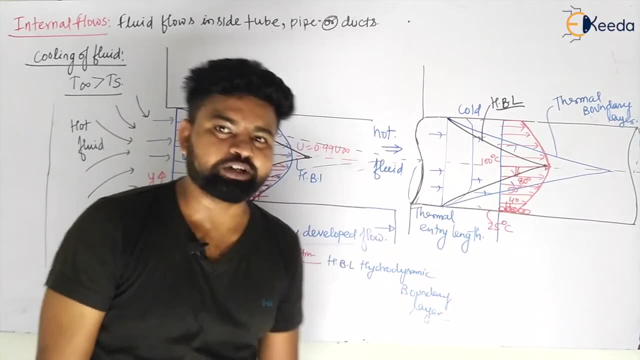 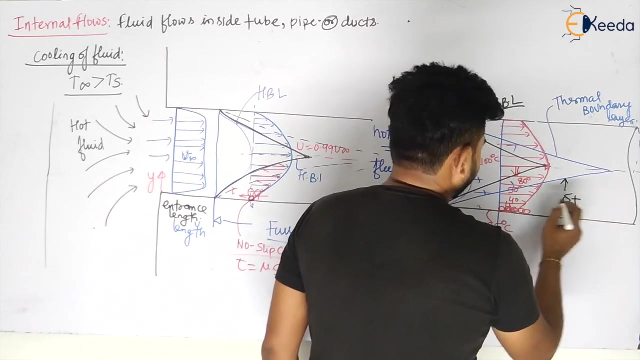 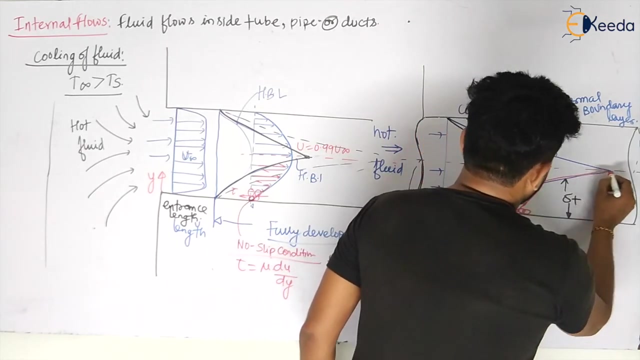 will be something like this, that will be your HVL. so like this these profiles will be developed, my dear students, and hope you have understood this again. you know that will be what that will be. delta thermal, my dear friends, delta thermal, let us take it back, take over like that, so you will feel the concept. 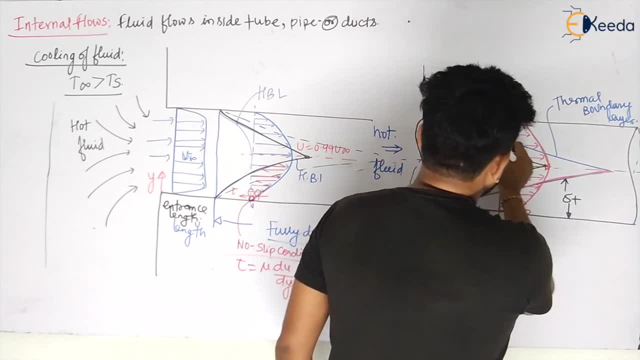 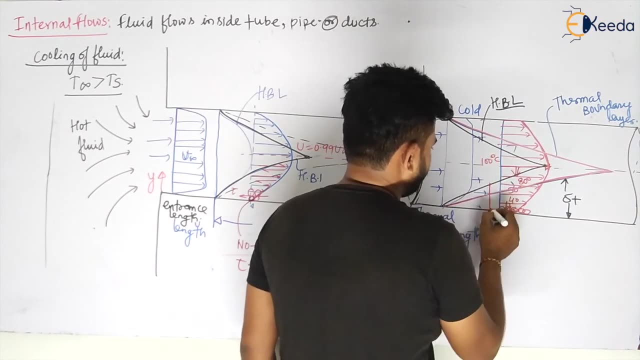 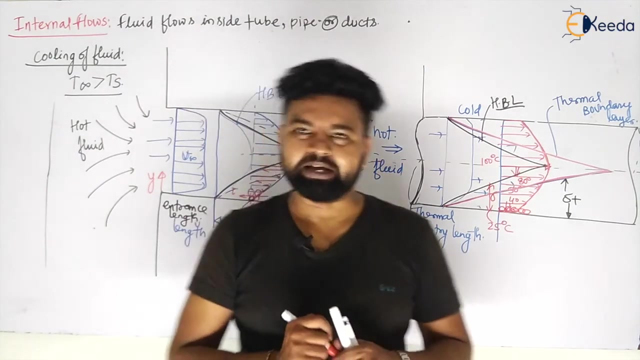 so this is your thermal boundary layer, my dear students, and for the black one, this is your hydrodynamic boundary layer, and you can calculate easily what del layer del, that is, hydrodynamic boundary layer- thickness. okay, so now this: the fluid will flow inside the pipes. let us analyze all these concepts now. so, when fluid is, 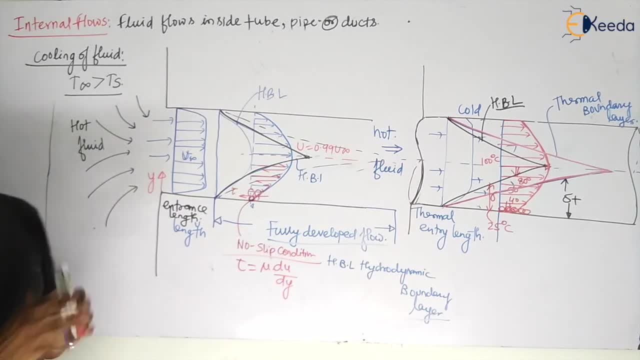 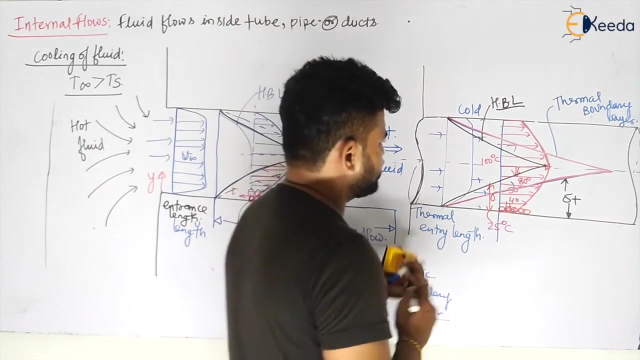 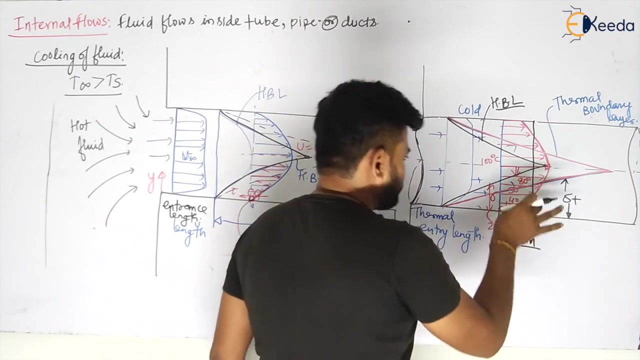 flowing inside the pipe. what will happen? let us see. let us see, my dear students. so we have not seen the mean temperature. so what will be mean temperature? you can easily calculate in this case also. so mean temperature will be something like this: that is Tm, this is constant. and what will happen? the mean temperature will 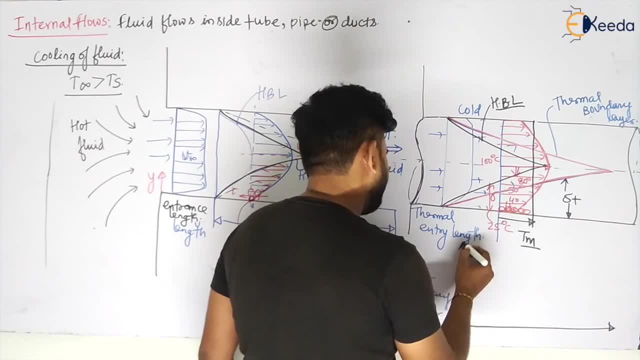 continuously decrease. now decrease or increase, if you will see the mean temperature. what is happening? this is cold, this is cold, and what will happen? the fluid will, like, lose heat continuously and due to which, inlet, the temperature of the fluid will be high. okay, and slowly, slowly, this. 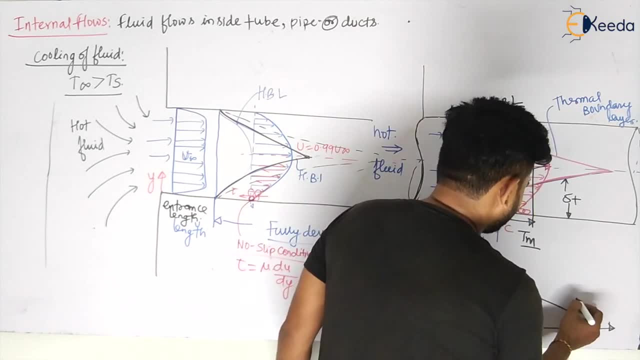 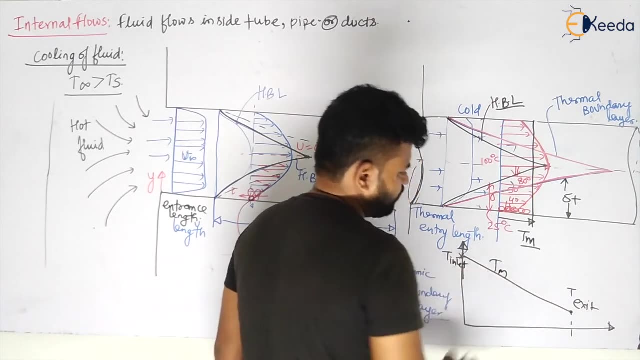 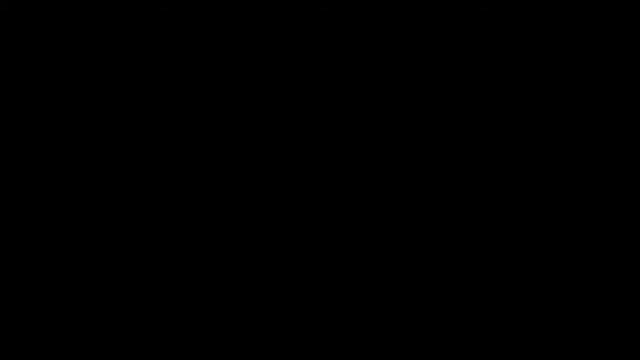 temperature will be decreasing up. to exit, my dear students, exit if this is inlet. so this will be your Tm profile, my dear students. okay, now let us see this. let us see. hope you have understood this well. this is that if Tm is very high. so that is what it was for our choice. all right there. 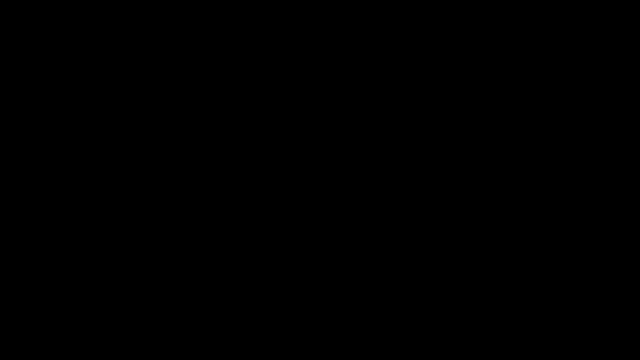 it was the whole forward. T spacing is equal to theocc semanas in dE and vaccine.